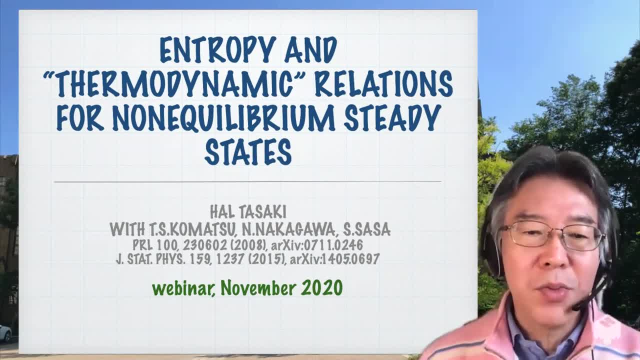 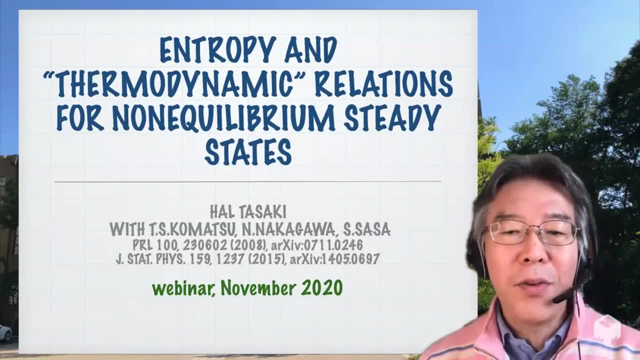 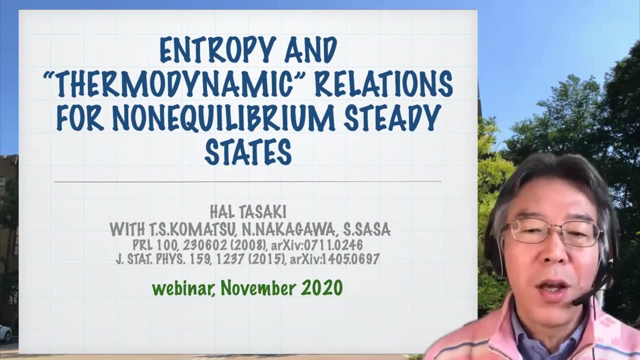 papers. we sort of believed that this work would lead to a new direction in non-equilibrium physics, But now I have a feeling that we were stuck at some stage. so no essentially new results. Nevertheless, I'm giving this webinar in 2020 because I still believe that there is something. 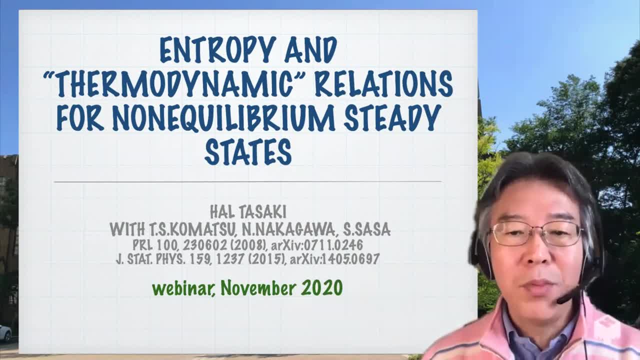 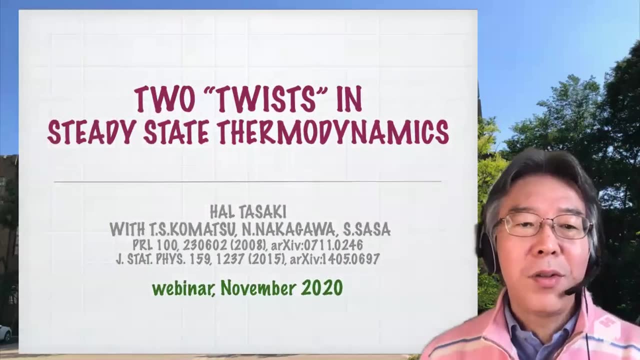 interesting in this work, And so I hope you will find it interesting, and I sincerely hope that you will come up with a new idea that will lead to a new breakthrough. Okay, so the talk has another title. I'm going to talk about two twists. 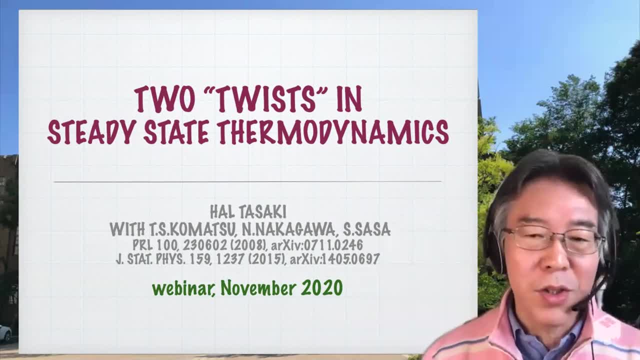 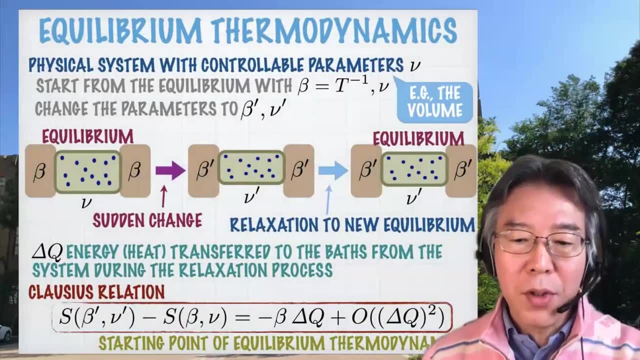 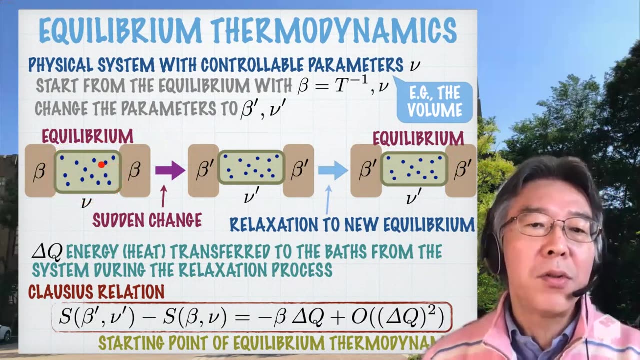 in steady-state thermodynamics, You will see what these two twists are. So motivation, Let me start from equilibrium thermodynamics, but which we all know about. So we consider a system which has a controllable parameter, nu, or the set of parameters nu, like the volume external field. 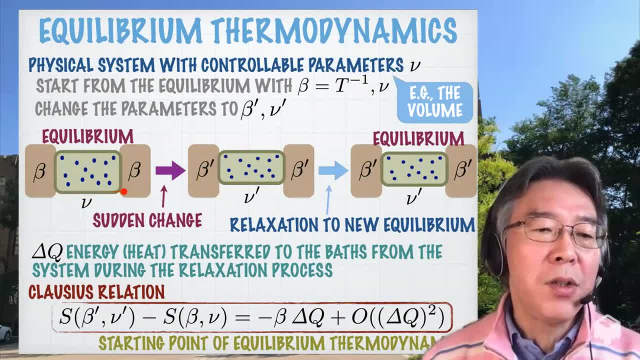 and something like that. And now assume that the system is attached to heat path, which must be huge, with some given inverse temperature beta. So you start from the equilibrium state with the inverse temperature beta and the parameter nu, okay, And at some stage we make a sudden. 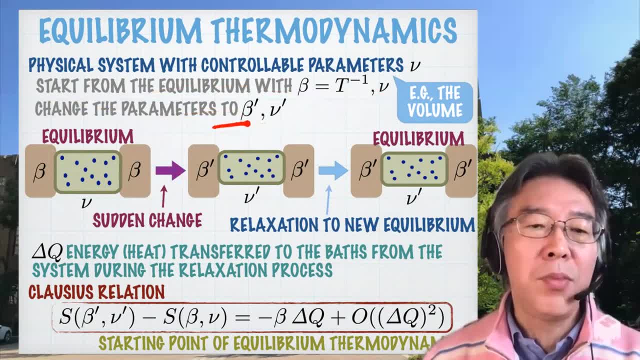 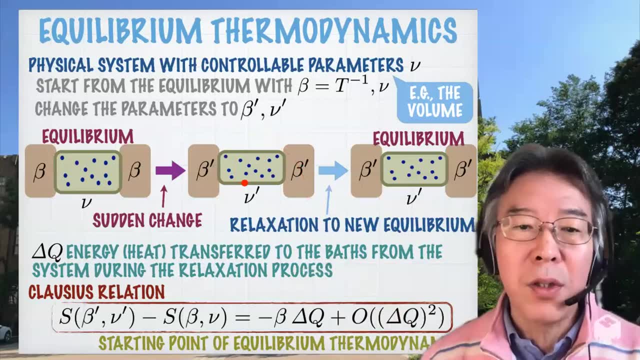 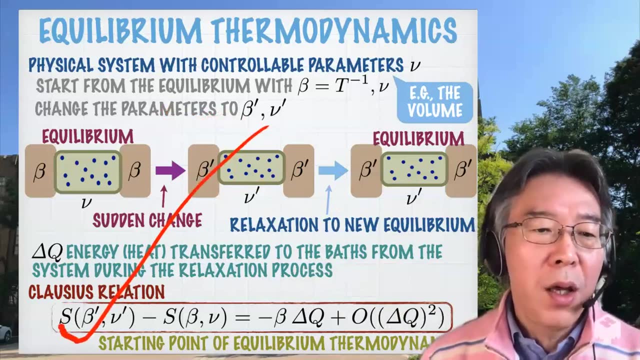 change of parameters- temperature and parameters to beta prime and nu prime, and then the system is no longer in equilibrium. But if you wait for a sufficiently long time, then of course it relaxes to a new equilibrium state with this nu, beta prime and nu prime And now by delta q. 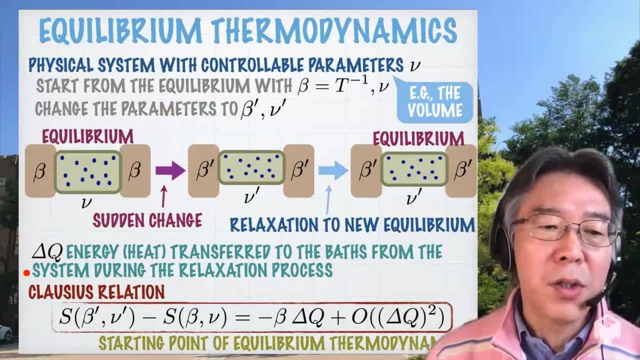 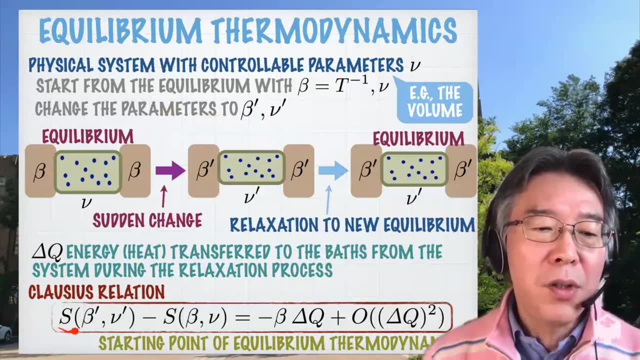 we denote the energy transferred to the bath from the system during the relaxation process. Of course that's heat. Then you know that the Clausius relation is valid. The difference in the entropies of the final and initial state is basically equal to. 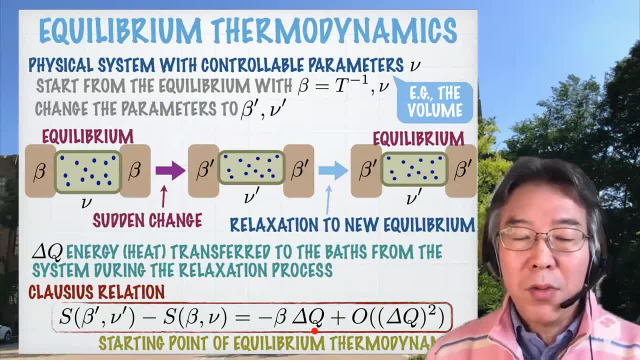 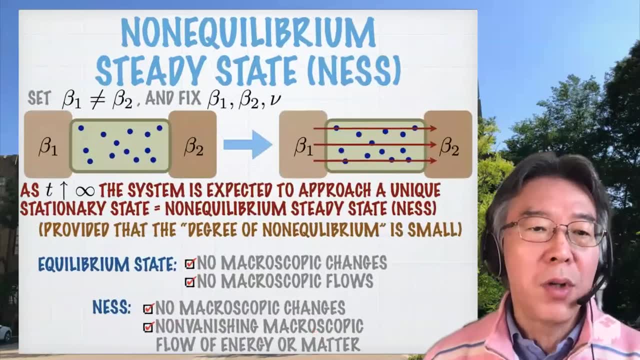 delta q divided by t. okay, So this, as you know, was the starting point of the whole theory of thermodynamics. Now I want to look at non-equilibrium situation. So, on the same setting, let's suppose that these temperatures of the bath are different. And now 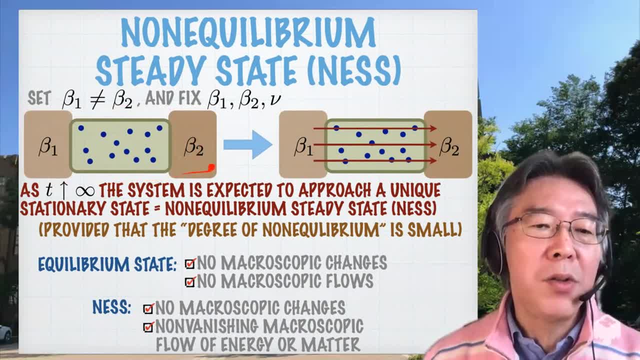 if you, you know, if you fix beta-1, beta-2 and the parameter nu, and then it is expected that, after the long time, the system approaches an unique stationary state, which we call non-equilibrium steady state. Nes, okay, And here's the comparison between equilibrium and. 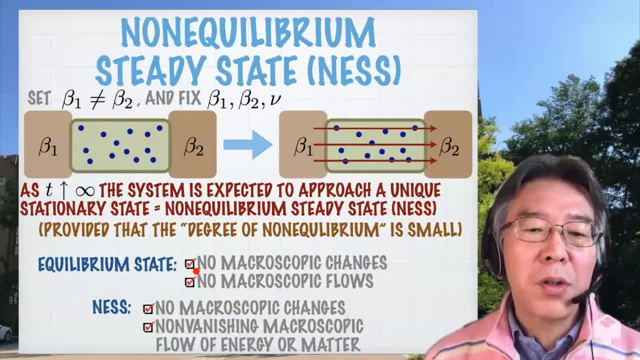 Nes, In both case we have no macroscopic changes at all. but in equilibrium state we have no macroscopic changes at all. And then what is non-equilibrium if we fix beta-1,, beta-2, and the parameters nu and? 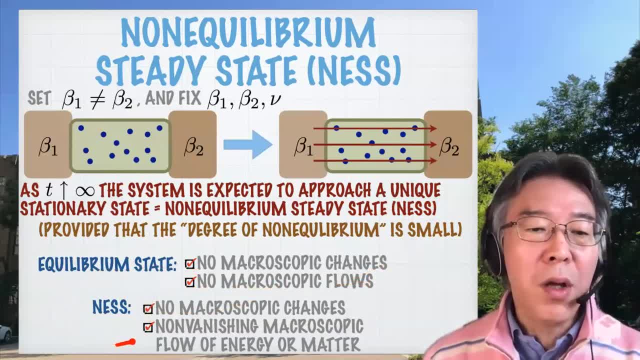 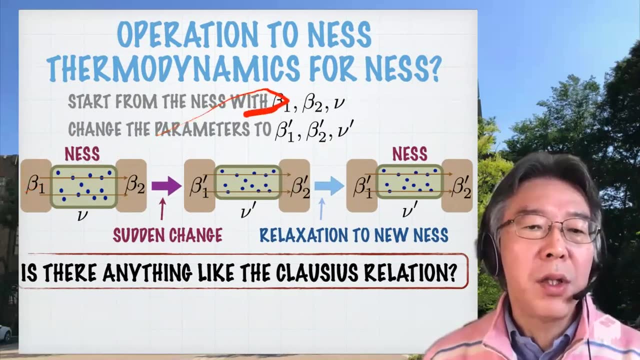 no macroscopic flows, But in NESS we do have non-vanishing macroscopic flow of energy or matter like here. Here heat is flowing Now, so suppose that we have a NESS with this temperature: beta one, beta two, nu. 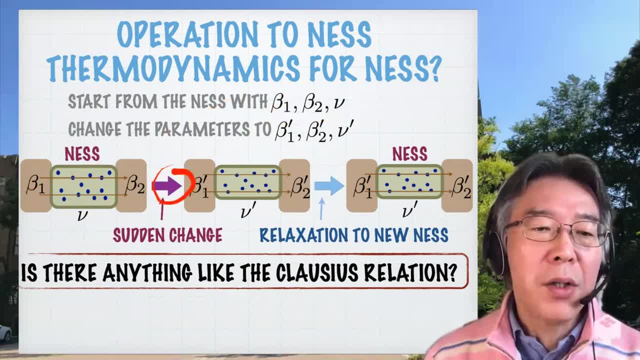 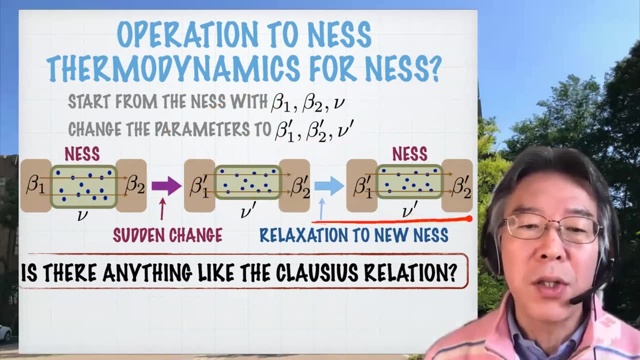 And, as in equilibrium case, we make a sudden change of these temperatures and parameters at some stage And of course the system is no longer in NESS. but if you wait for a sufficiently long time, you expect that you will reach another NESS, new NESS. 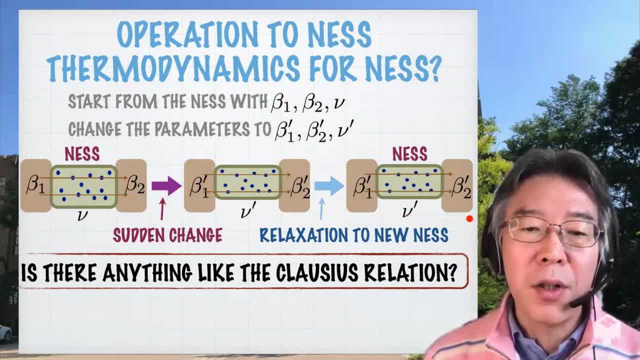 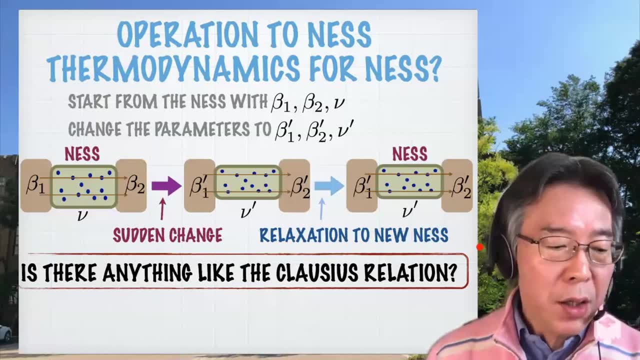 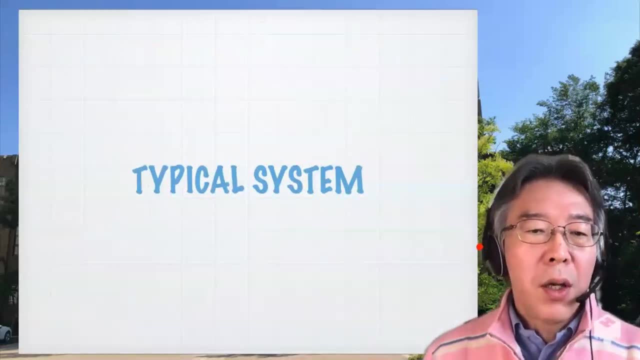 And now we want to ask: is there anything like the Clausius relation associated with this non-equilibrium relaxation process? And the main result of this talk is a derivation based on general microscopic models. So a typical system we are looking at is a system. 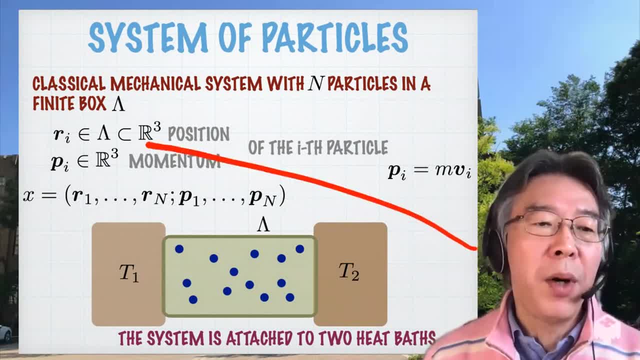 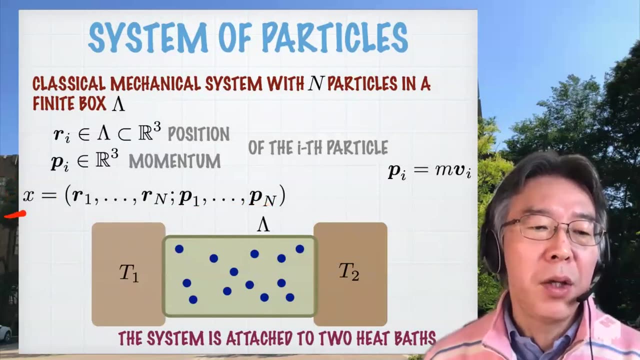 of N, classical particles confined in a box, And by RI we denote the position PI, the momentum of the ice particle, And by lowercase X we denote the collection of all the positions and momentum. Okay, so this is a huge, big quantity. 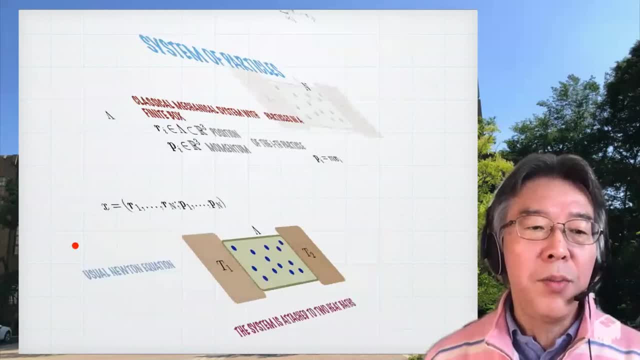 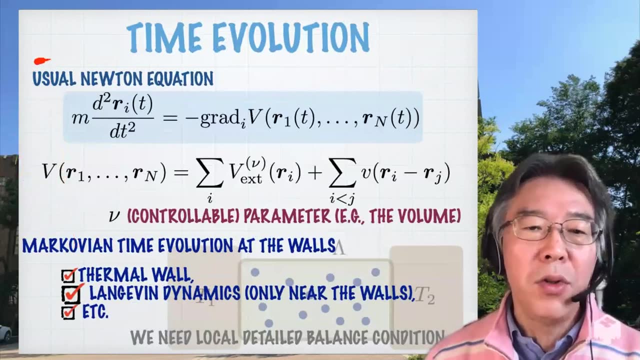 And we assume that the system is attached to two heat paths. So the time evolution of the system is described. So the time evolution of the system is described. So the time evolution of the system is described by two parts. One is a usual Newton equation with potential V. 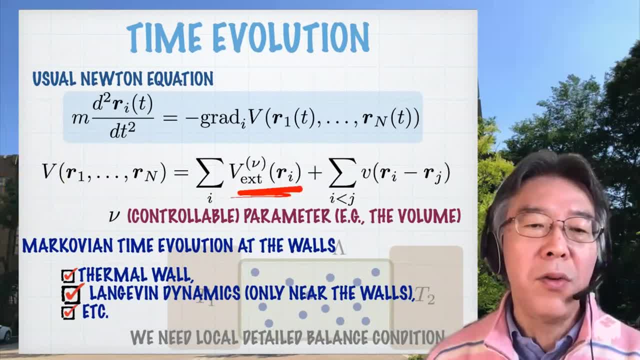 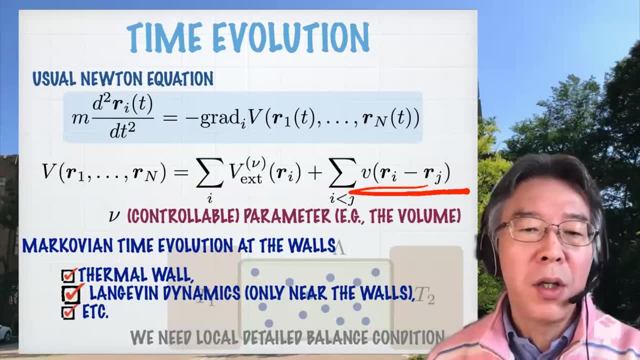 And we assume, for simplicity, that this external force potential contains this controllable parameter like external field volume or whatever. And here's two: body interaction. Okay, but this can be almost anything. And this is deterministic part And the stochastic part here. 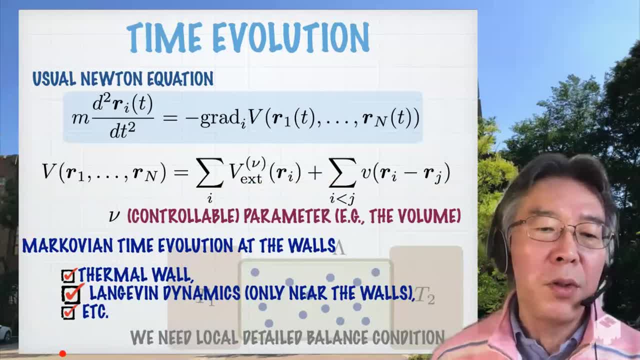 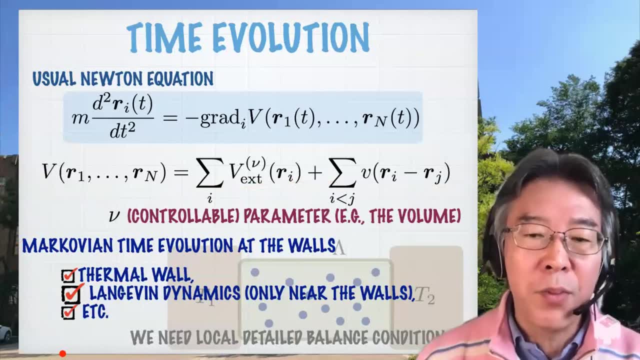 we have stochastic part, which is basically Markovian time evolution, which describes the you know, which describes the. you know the effect of the walls having temperatures T1 or T2.. the effect of the walls having temperatures T1 or T2.. 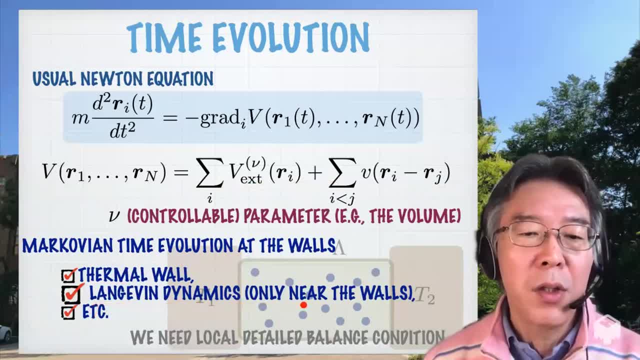 So the most standard thing is to use Langevin dynamics only near the walls, And or you can use something called thermal wall that I'm going to explain in the next slide, or anything else. But the only assumption we need is that this Markovian time evolution satisfies. 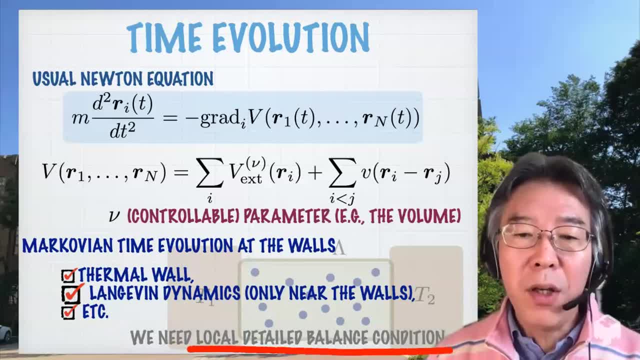 a local detail balance condition. This is a very standard terminology in non-electronics. This is a very standard terminology in non-electronics, So you can find it in any reviews or many papers. So you can find it in any reviews or many papers. 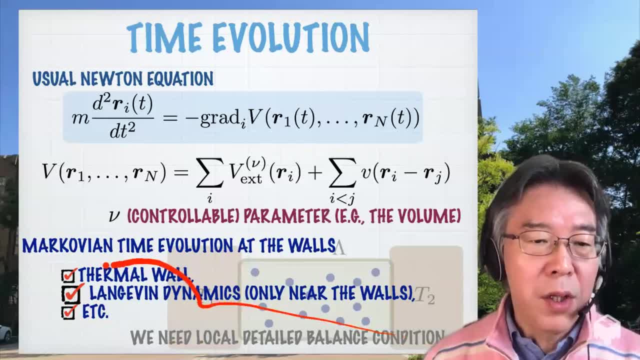 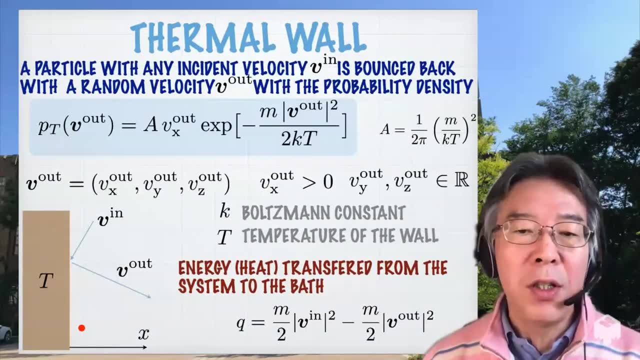 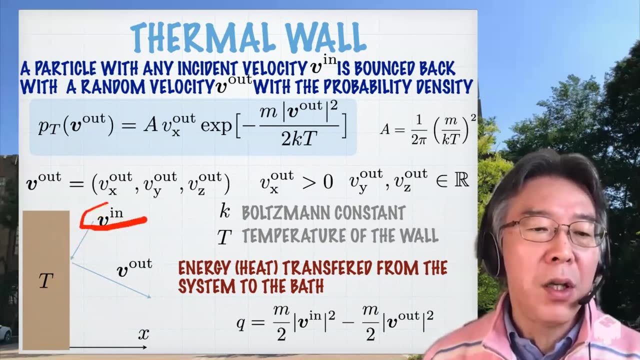 Okay. So, and all of this satisfy local detail balance condition. So, and all of this satisfy local detail balance condition. Just one word about thermal wall. It's an especially designed wall which describes the body with temperature T, So whatever the initial velocity of the particle is, 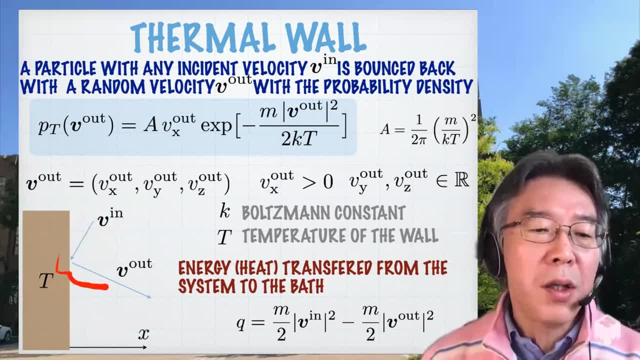 it forgets the part, the velocity, and it's. it will come out from the wall with a new velocity, v out, which obeys this probability distribution. then this describes the effect of wall with temperature t. this is standard and also here note that you can compute this energy difference and this can be interpreted as the microscopic. 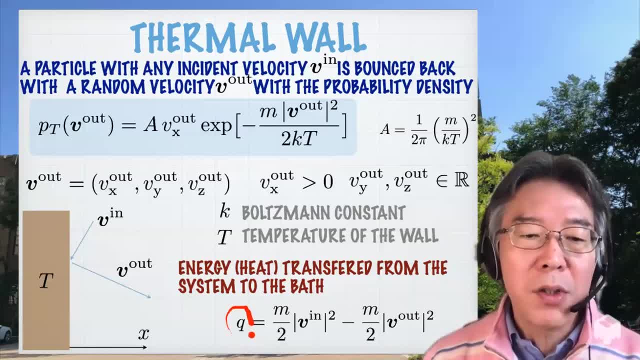 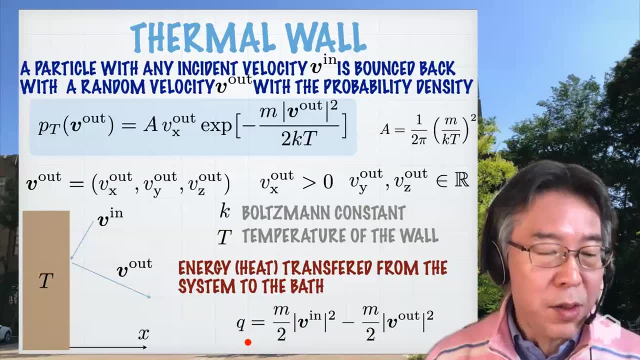 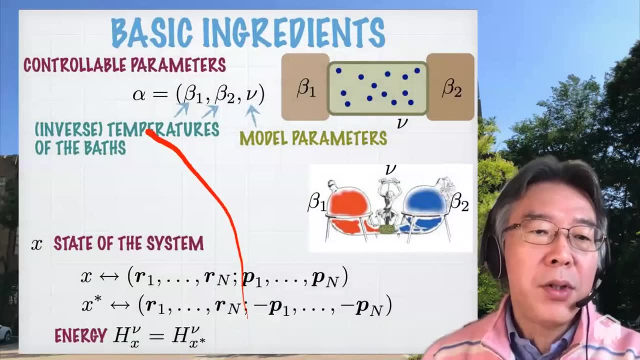 heat transfer from the system to the bath. so if you sum this q up, you will get the total heat. okay, or you can compute heat current and so on. that's important general setup okay. so these are permitted parameterization. so the control permit we denote by alpha the 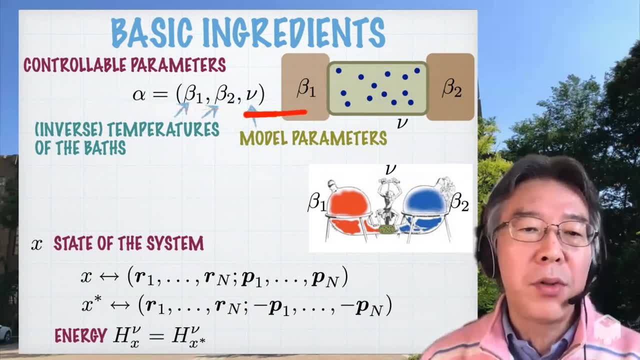 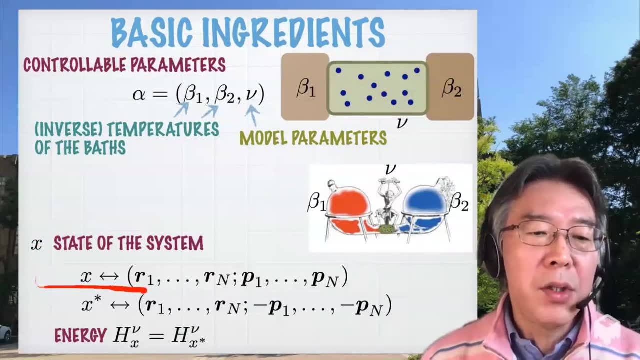 collection of two inverse temperatures between beta 2 and this model. parameters like the volume or the external field, it's like this- and x. the state of the system is this, and this is important: by x star i denote the time reversal of x. so at r are the same, but you uh, reverse all the momentum, okay, and we assume that the energy of 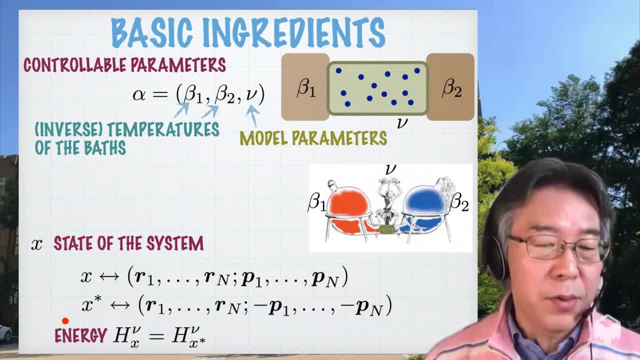 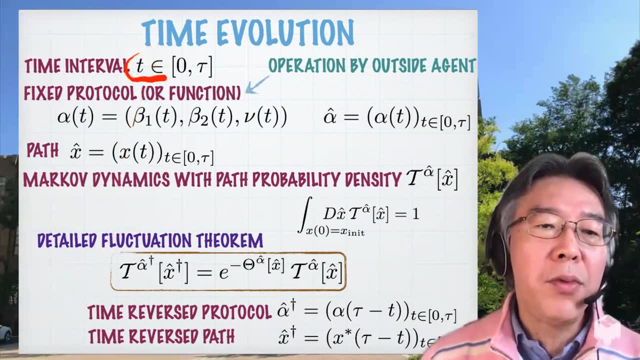 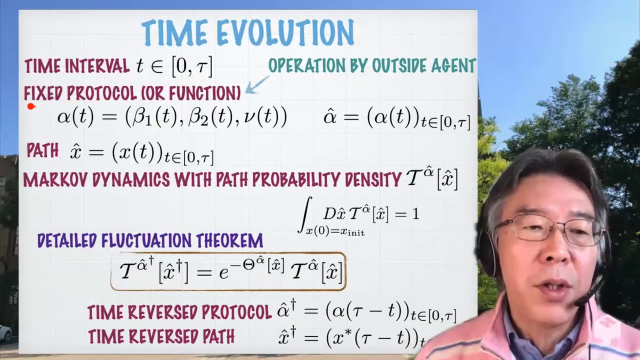 the system is invariant under time reversal and here comes time evolution. t is the time variable which runs between zero and tau. tau is a big quantity which is fixed, and this is a basic, important assumption. i assume that this alpha t, alpha parameter is a function of temperature. that means beta 1, beta 2 and nu are functions of temp of time. i'm sorry. function. 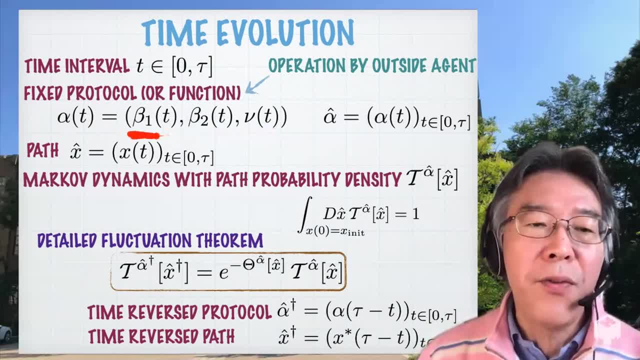 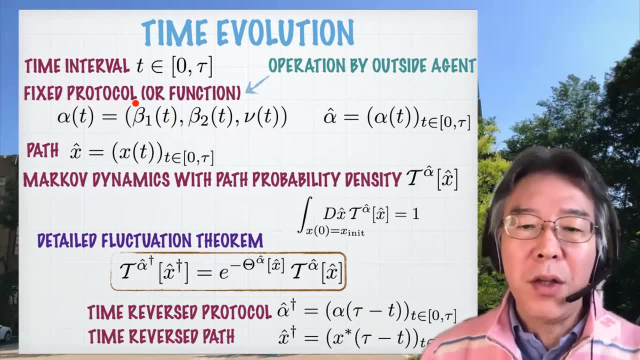 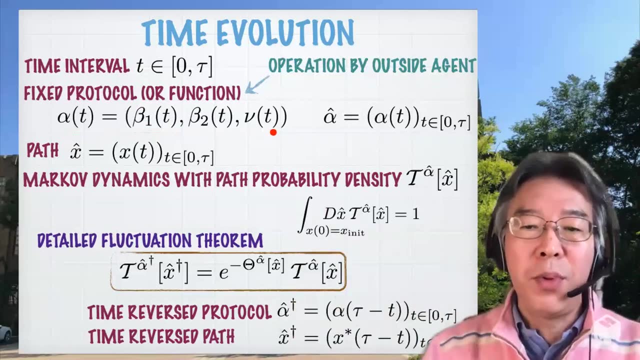 of time t, and these functions are fixed before the experiment. so that is usually called protocol. so before running your experiment you did you decide how you change the temperatures or how you change the volume and so on, and you probably program these changes. that's called protocol, and you know. then experimental setup. 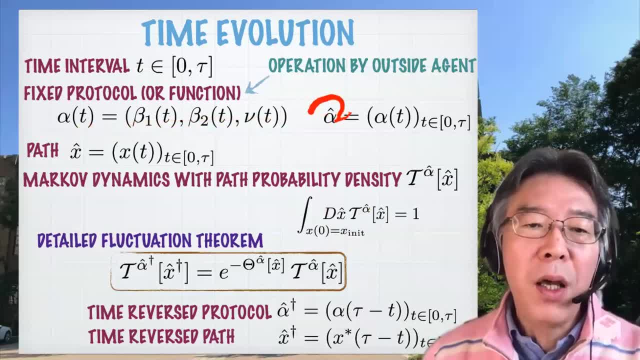 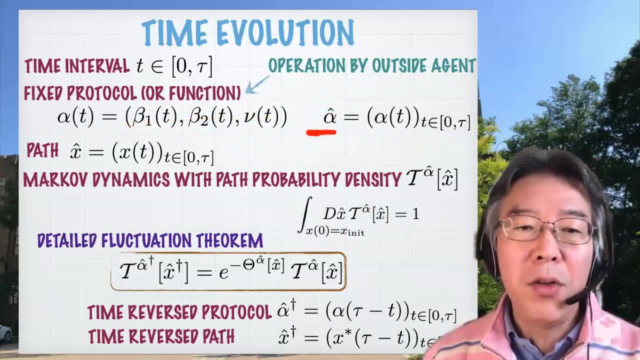 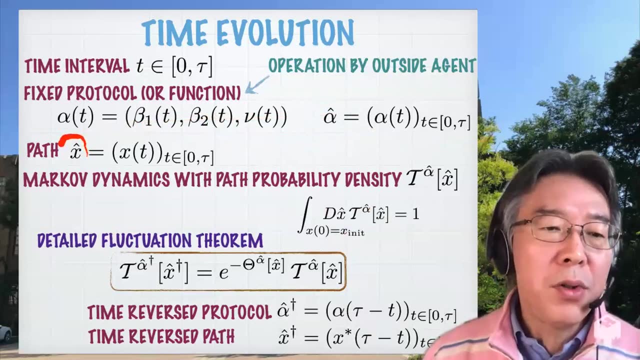 simply just obeys this. and by alpha hat i denote a whole function. okay, and so this is something you decide and you determine. on the other hand, x hat is something uh system determines by solving the equation of motion, and also it's stochastic. okay, when by x hat i denote the whole path. 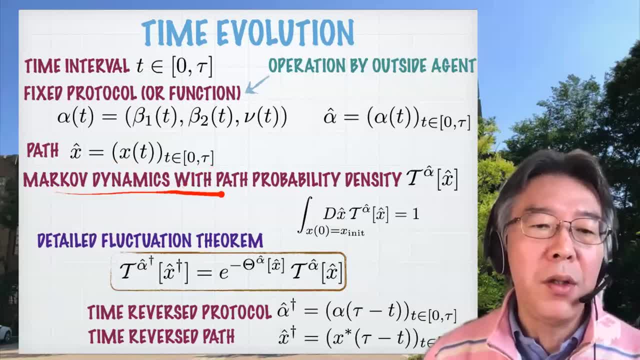 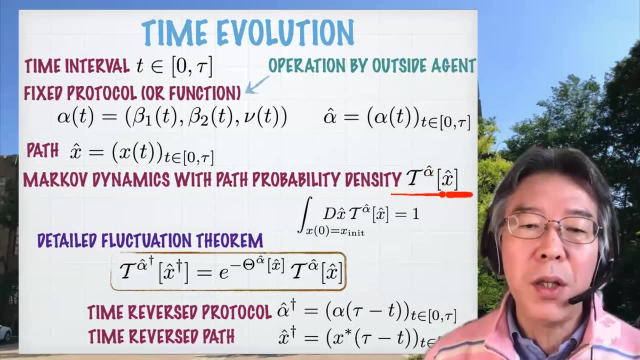 and then, uh, since the dynamics is markovian, you get, uh, you get something called the path, probably density for each realization of path, which of course depends on alpha hat. okay, and so this roughly tells, roughly speaking, this is a probability that you get a specific path, x hat. 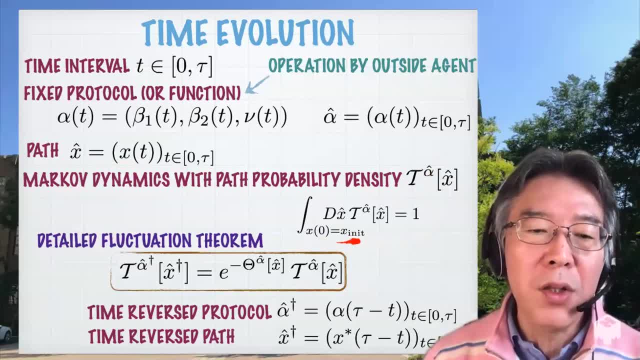 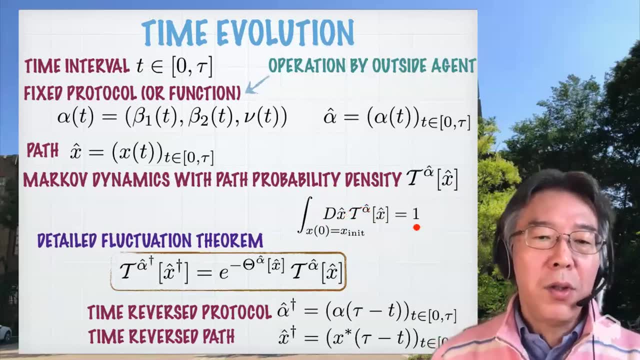 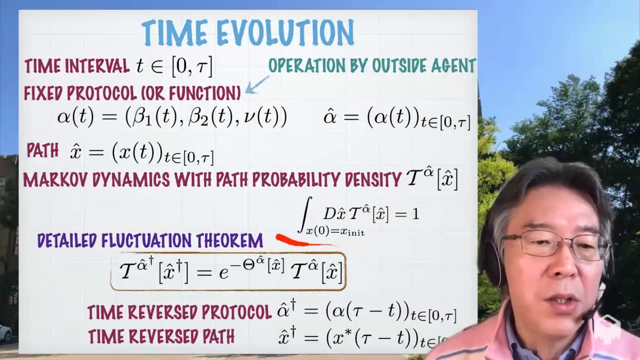 and it's normalized in this way. so if you fix the initial condition and sum up over the path- i'll sum up over all the paths- then you get one okay. so again, this is a standard object and i say that this t? uh path probability density satisfies a very interesting symmetrical detailed fluctuation. 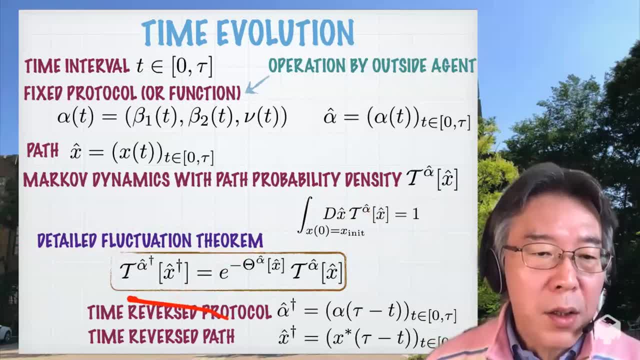 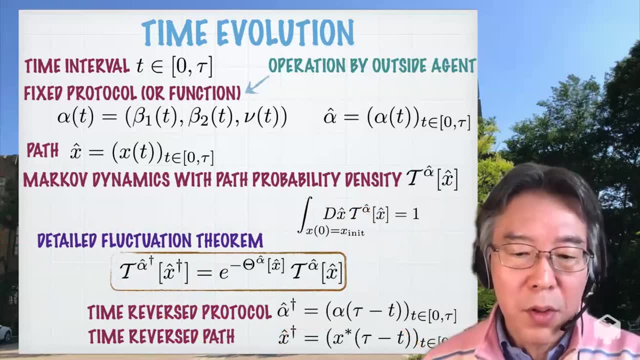 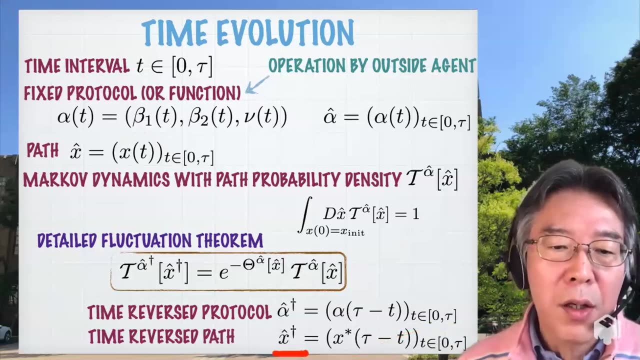 theorem and here, uh, i have new notation: by alpha hat the guard i denote the inverse protocol, inverse protocol in simply, the time is, time goes in the opposite direction here, and x hat the guard is the inverse path, the reversed path, and again time goes backward and also i take this time reversal, okay, and then i i say that this equality is valid and for this, uh, 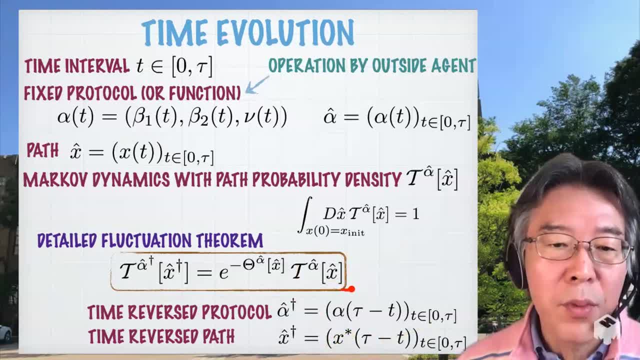 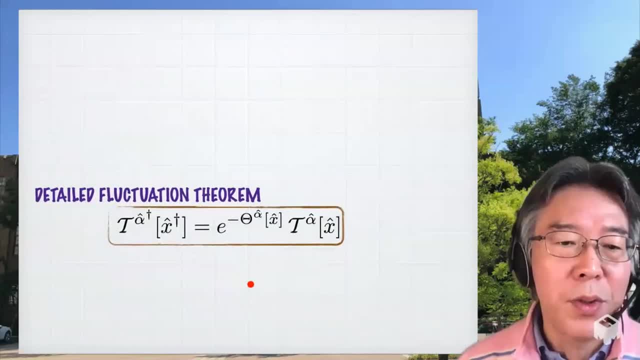 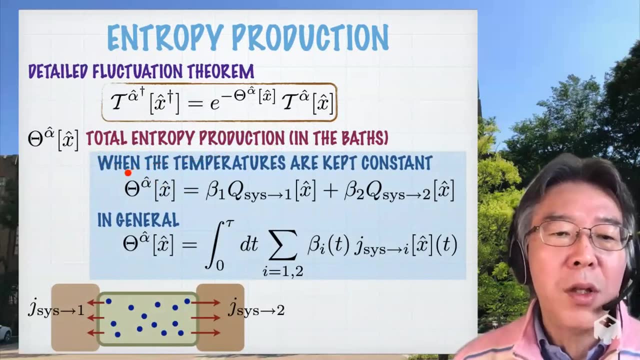 probability density for the forward path and probability density for the backward path, and. but here you have some new quantity that i have to explain. uh, this theta here is called the total entropy production in the bath. uh, in the simpler case, when the temperatures of the baths are 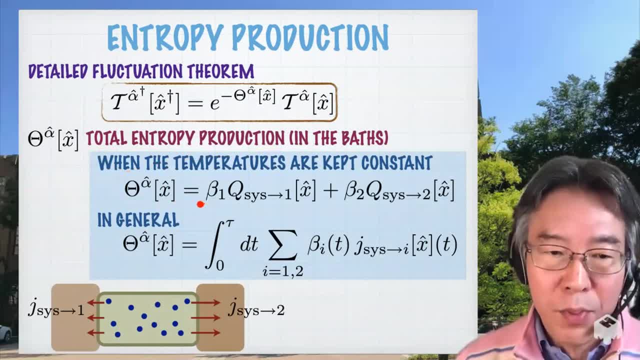 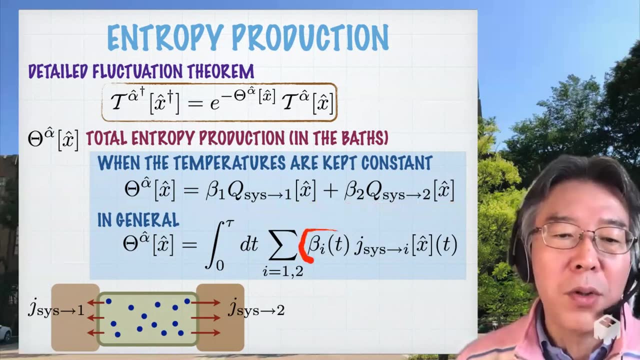 kept constant. it's simply the total entropy production. so q from system to one is the total amount of heat that the best one absorbed during this process. so this is the entropy production. and this is for the second thing and in general, when the temperature of the best is time dependent. 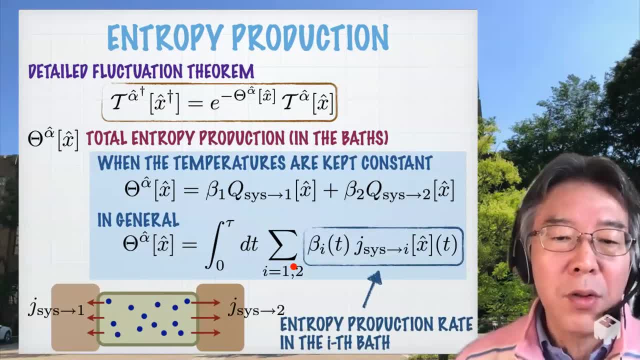 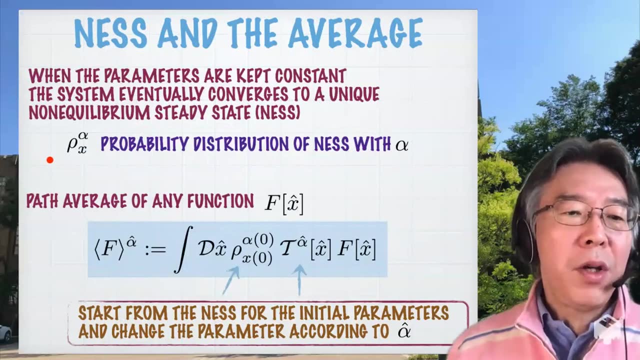 and then you consider this quantity, which is entropy production rate in the ice bath, and you simply integrate. okay, by this way you get the total entropy production in the bath. and this is the time of quantity we want we are looking at. first of all, we assume that when the 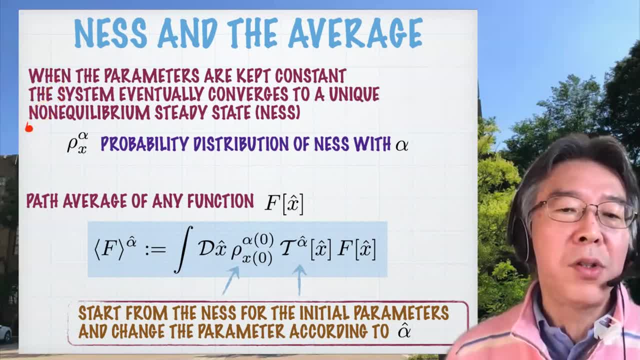 parameters are kept constant, the system eventually converges to a unique non-equilibrium steady state nest, and i denote by rho alpha of x. alpha is the parameter, x is the state of the system. probability distribution of nest with parameter alpha. okay, now suppose that we are interested in. 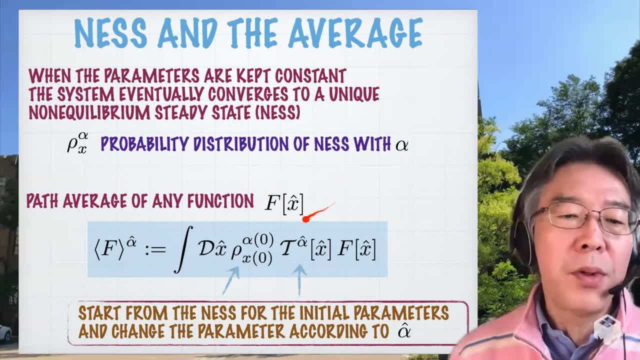 any, any function f of the path, okay. and then we consider this time average, uh, this average which depends on this, which depends basically only on this, uh protocol alpha hat. what is this? well, it's here you start from the nest. for the initial parameters, alpha zero, okay. 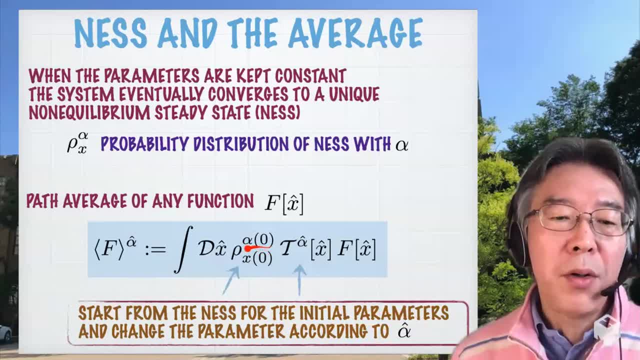 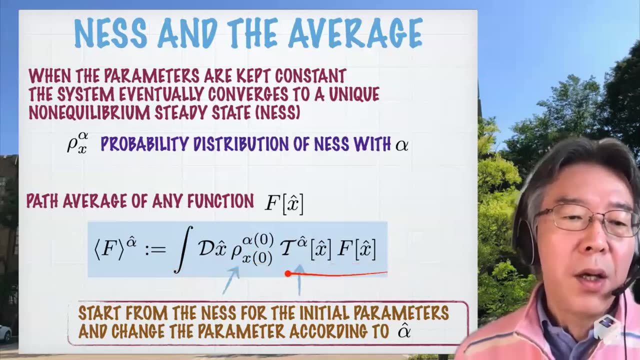 so you are first. first you are in nest with parameter alpha zero and then, uh, you start your protocol and you start changing your alpha and the system changes, the state of the system changes according to this, and then you simply average. okay, so yeah, you start from the nest with alpha zero. 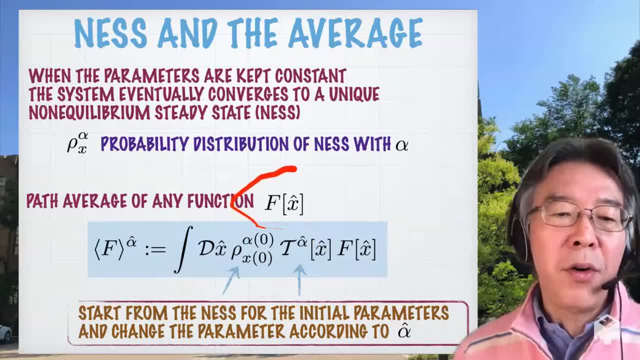 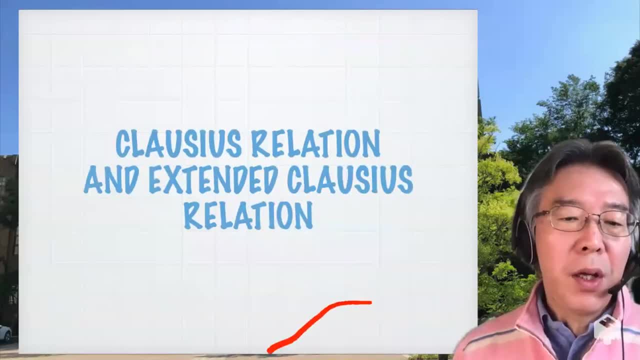 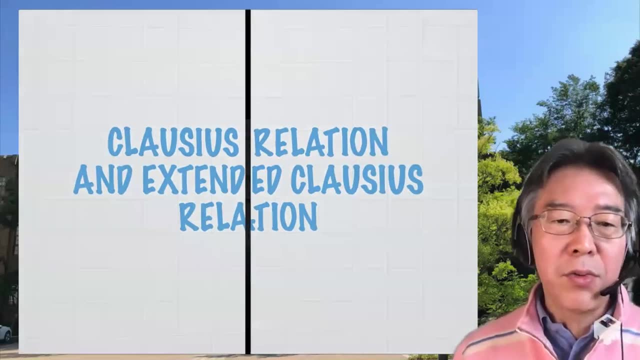 and just do your protocol and consider the average of any function f of the path. okay, so that's a basic setting, and now i'm ready to talk about the closest relation, the original closest relation and the extended closest relation of hours. so this is the equilibrium case that everybody know already. 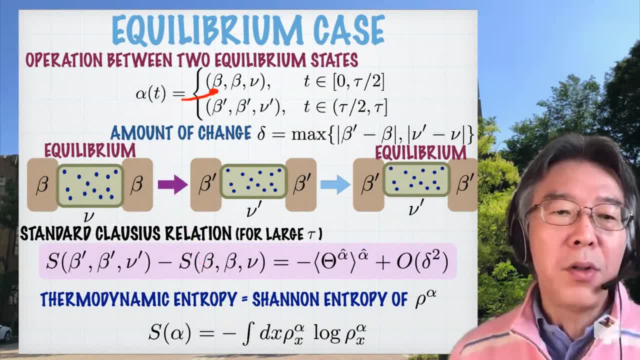 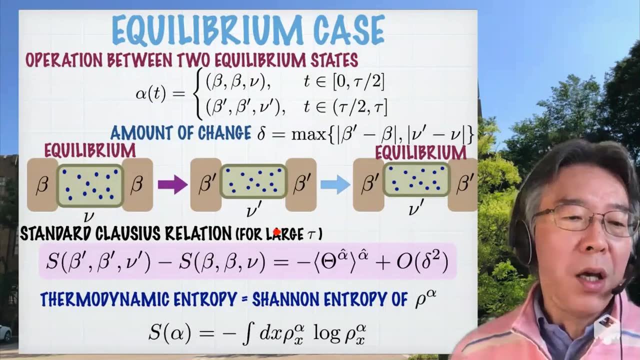 know. so this is a simple step protocol. you start from beta, beta, new, the temperatures are the same, so this is equilibrium condition, and at some stage you change it to beta, beta, prime, new, prime okay, and delta denotes the amount of change, and then, in this case, uh, for large enough tau. 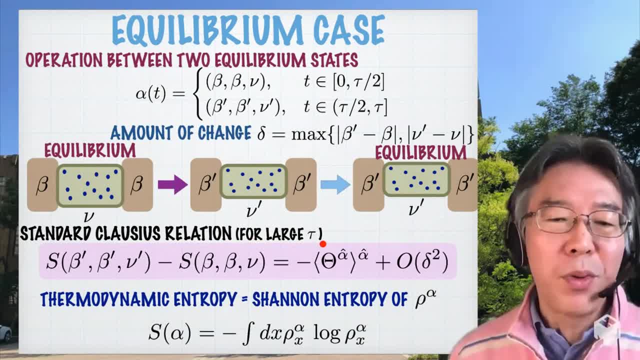 we can prove, or many people can prove- this was proved many, many times uh- that the difference in entropy is equal to the minus of the total entropy production in the bath. and here the entropy is just thermodynamic entropy. it's a Shannon entropy of rho. in this case, rho is just a canonical distribution, so it's a very standard thing. 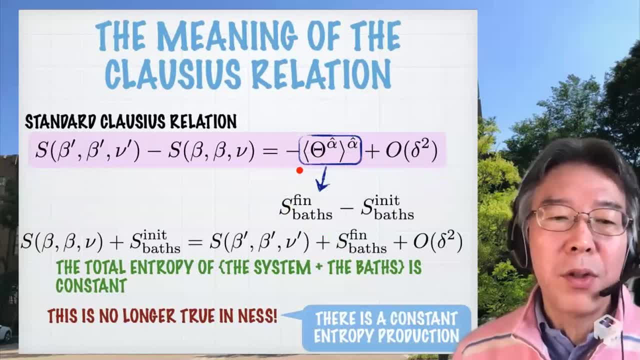 and in this case- uh, this is, this- has a simple interpretation. so this is a total entropy production. so it means that this is a difference of the total entropy production and this is the initial entropy of the final entropy and the initial entropy of the bath. so this equality can. 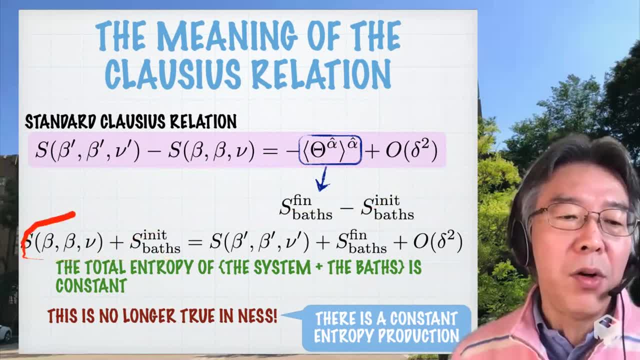 be rewritten in this way. so this simply tells you that this is an initial entropy of the system plus path and this is the final entropy of the system plus path. okay, with some minor error coming from this step protocol. so this simply says that the total entropy is constant, but i will say that this 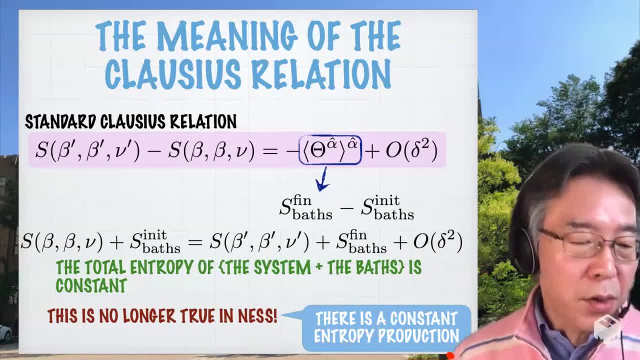 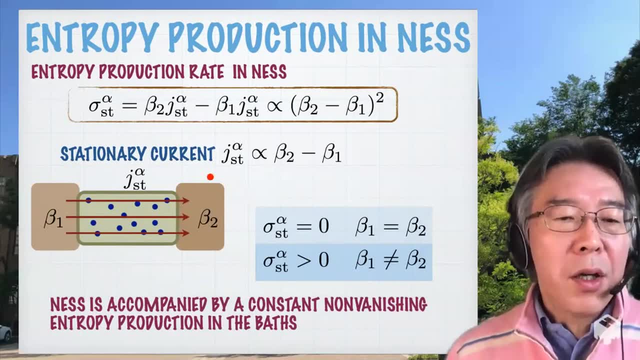 is no longer true in this, because we have a constant entropy production. what is this? well, so consider a steady, non-equilibrium steady state in this. so we have this steady situation with steady heat current which is proportional to the temperature difference, and now, uh, this is the entropy production rate, uh. 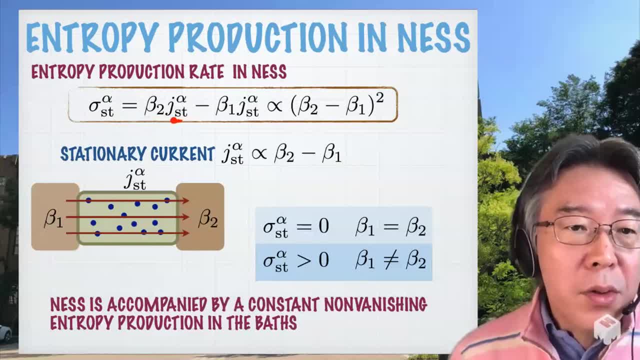 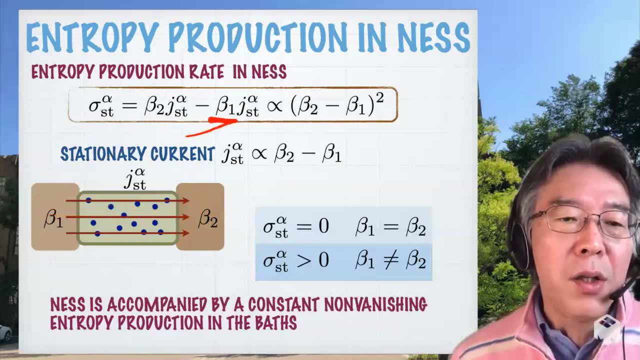 beta 2, j stationary. this should. yeah, this is the entropy production in this path, and the heat is going in the other, in this direction. so this is the entropy production in the first path. and now, since j is proportional to beta 2 minus beta 1, this entropy production is proportional to: 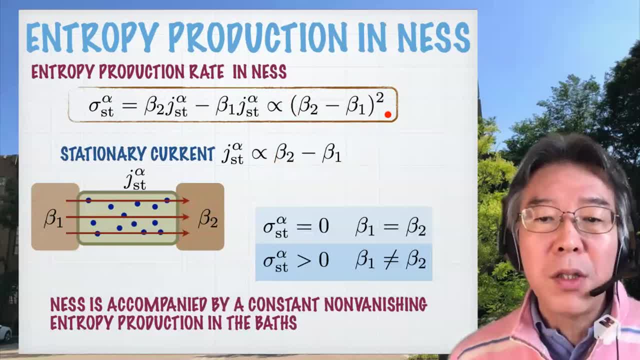 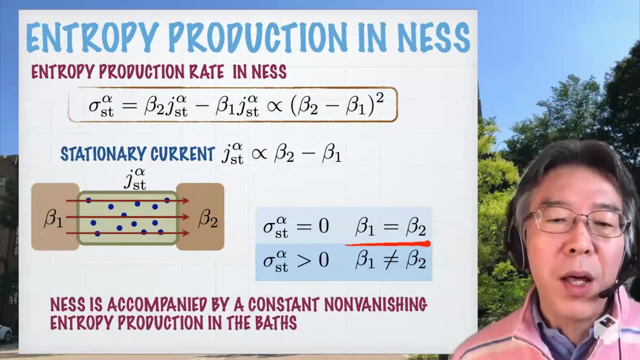 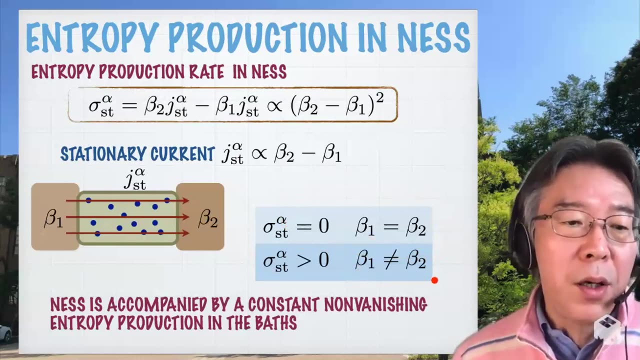 the square of the temperature difference. that means it's strictly positive. this means that the entropy production rate is zero only when the temperatures of the two baths are the same. this is equilibrium case, and it's strictly positive whenever the temperatures of the two baths are different. so ness is accompanied by a constant, non-vanishing entropy production in the 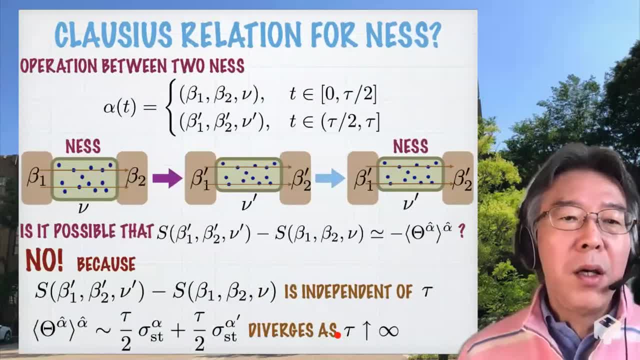 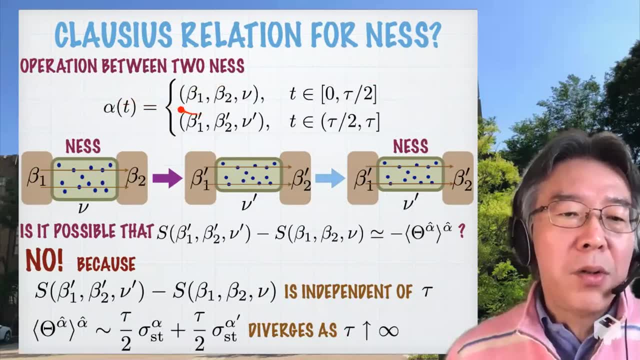 bath. that's very important. now i ask if there is like something like clouds, isolation for ness. so let's consider this step protocol that we considered before. uh, first we have our parameter is beta 1, beta 2, new and at some stage at time, tau over 2, we change the parameter suddenly to beta 1. 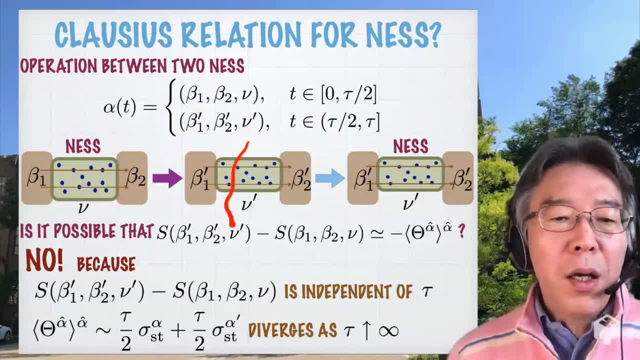 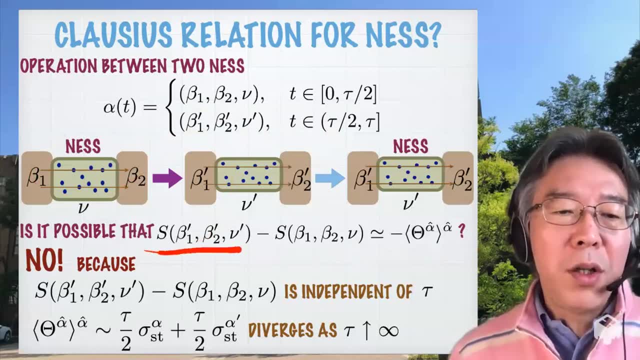 prime, beta 2 prime, new prime, okay, and now we ask: can there, is there, is it possible that we have this kind of relation? so we don't know what these are, the what, what this entropy, entropy is, this is a non-equilibrium entropy, uh, but can we ask if, if there's, if, is it possible to that this kind of? 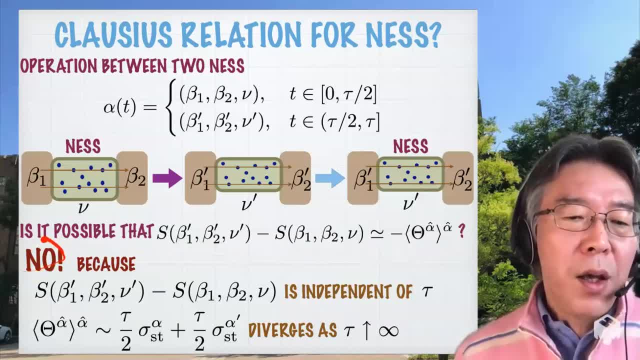 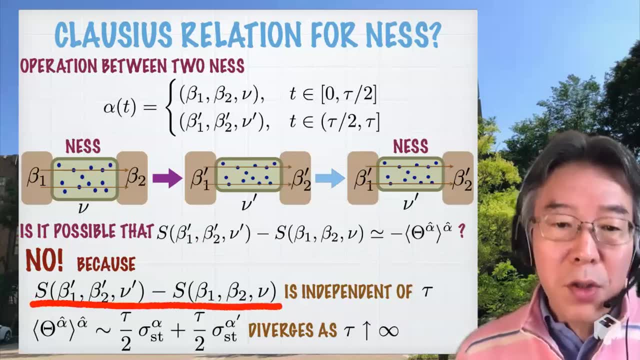 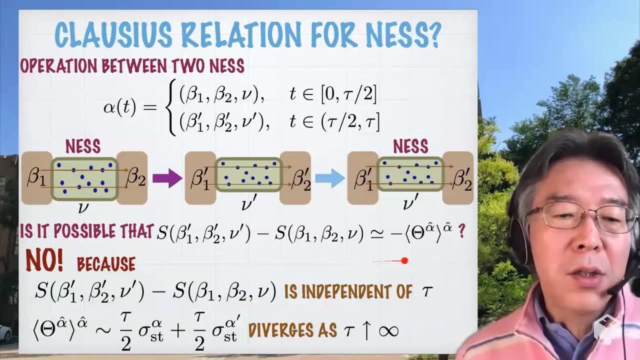 relation is valid, but the answer is definite: no, because whatever. whatever this non-equilibrium is, this is simply the difference of the two entropies into ness. so this difference is, of course, independent of tau. but here on the right hand side, you have entropy production total. 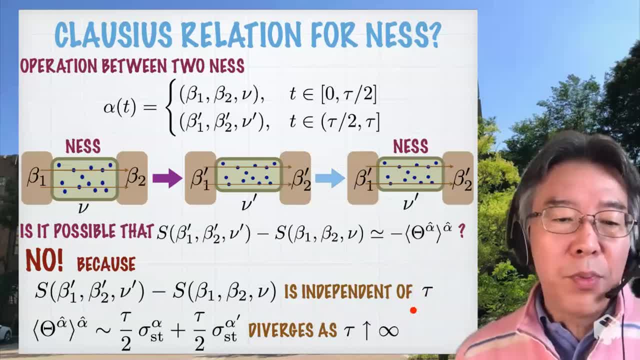 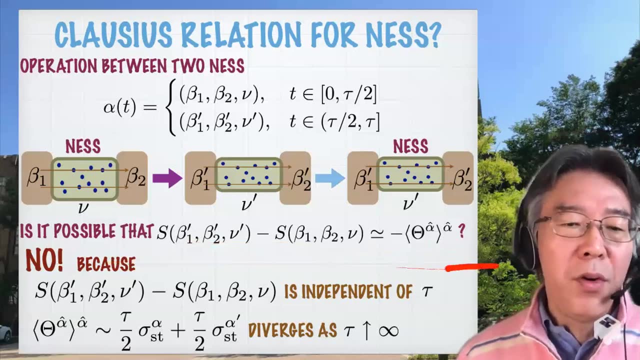 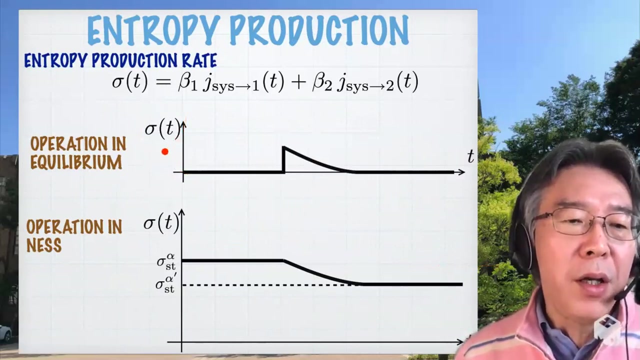 entropy production. so, since we always have entropy production in ness, this guy is proportional to tau and diverging in tau. so this is independent of tau and this is diverging in tau. so never, we never have this kind of relation divergence. so this is a schematic picture. uh, this is a entropy production rate and this is a case of. 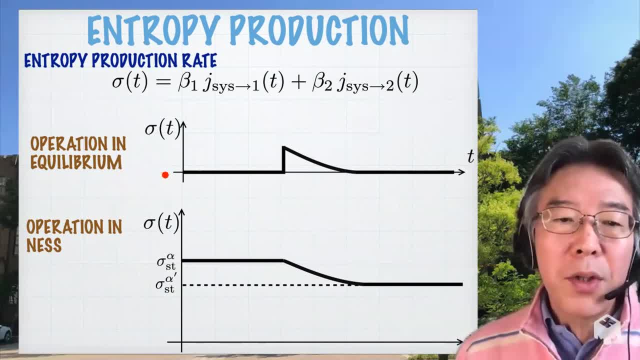 operation in equilibrium. so in equilibrium case we start from equilibrium, so the entropy production rate is zero. and then here you make this uh operation, so the system is no longer in equilibrium, so you have non non-zero entropy production, but again relaxation process and again the entropy production becomes zero. 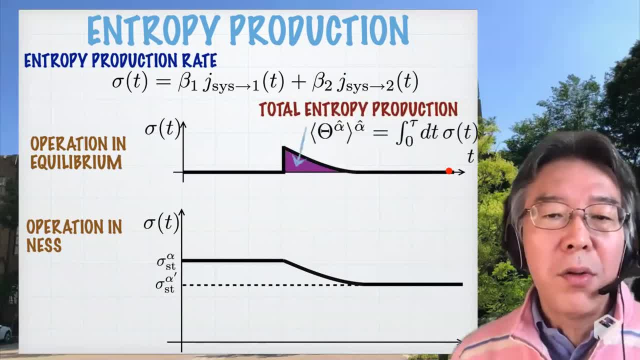 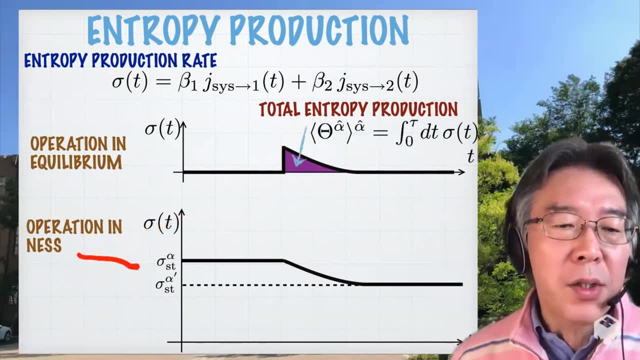 so, uh, in this case, if you integrate, over integrate this quantity, you get something finite. this is the total entropy production. now, this is a case of ness. you start with a nurse, so nothing, no operation, everything is steady. but you always have non-zero entropy production. here you make operations some. 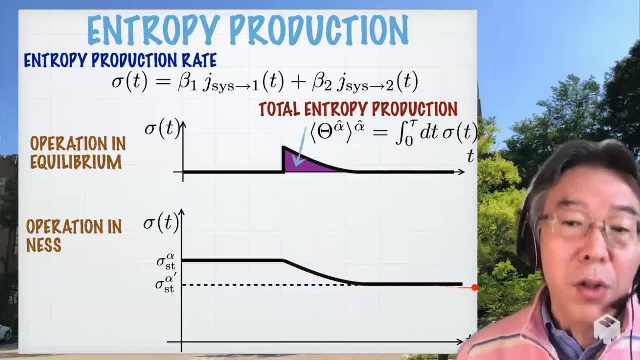 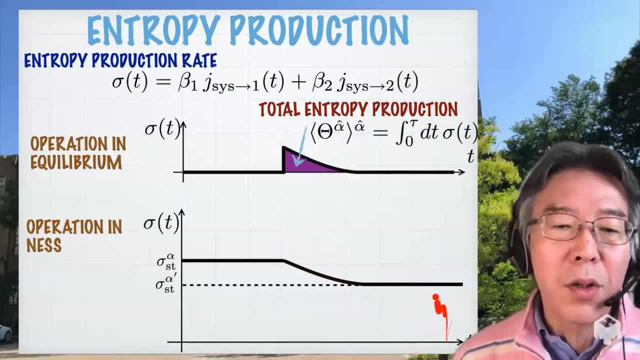 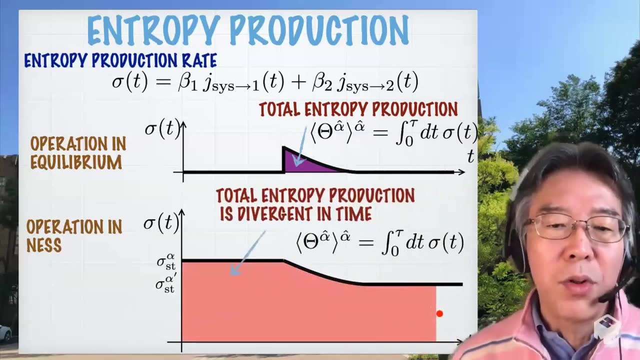 relaxation process. here system has relaxed to a newness. no, nothing changes against steady, but still you have to pay this amount of entropy production rate. okay, so you always have to pay some amount of non-term entropy production rate. so if you integrate this, of course you get some diverging. 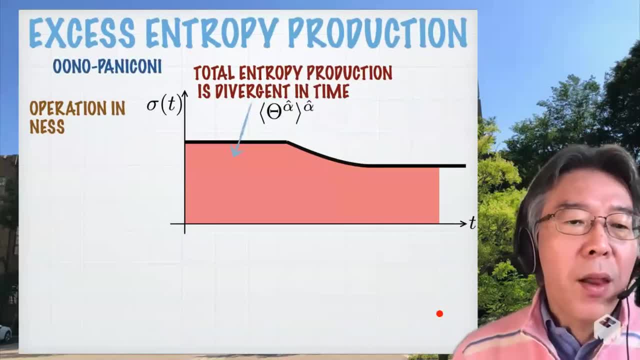 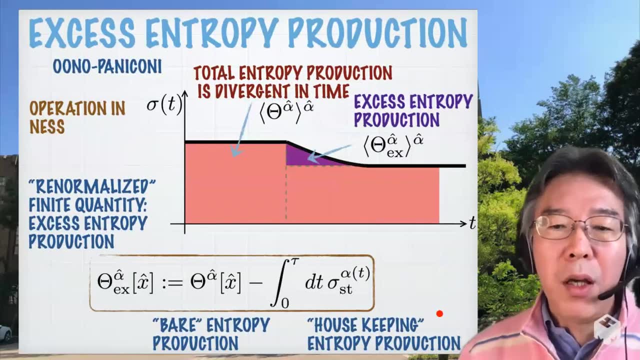 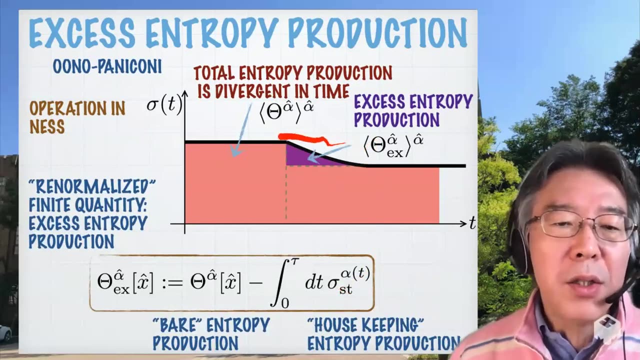 quantity. what shall we do? well, so this is a diverging quantity. so, uh, what we learned is that whenever you have a diverging quantity, you subtract something, renormalize to get finite quantity. in this case, it's very natural to subtract the area of this part and consider only this thing and this, uh, the remaining. 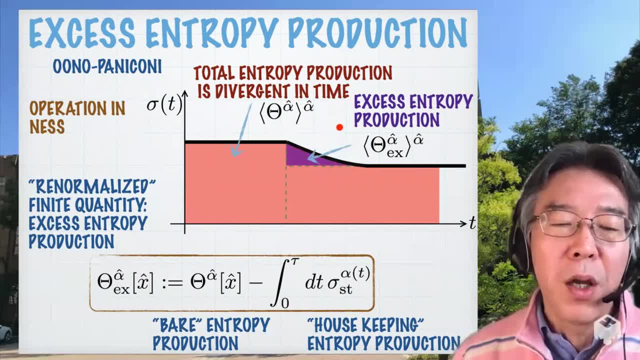 finite quantity is called excess entropy production. what did we do? well, as, as i said, uh, when, if your parameter is alpha prime, you know that you must at least pay this amount of entropy production to maintain this steady situation. here you don't have anything steady, but here you have a steady. state and we know that in order to maintain steady stable state over time you need something that is so steady and � Does that mean when it is alpha prime you need to add an existing component? So by doing this you get a steady state but of course you don't have nothing steady but you on doing e. so we make any kind ofожно and when you show this method we use, we used data to tell you the Sockey wheel, respect that, the floor pressure that there gives us as a student marker, which is the different Δ, and how much��운 it is actually. 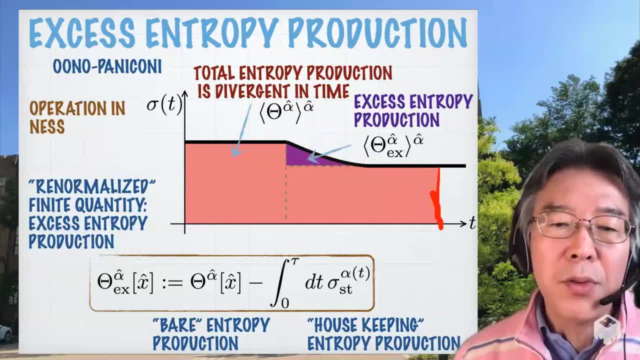 steady state with this parameter, alpha prime, then you have to pay this amount. So we know that we have to pay this amount, So you simply subtract this. And here this is the amount that you have to pay. so you subtract this, So we are left with this finite quantity. 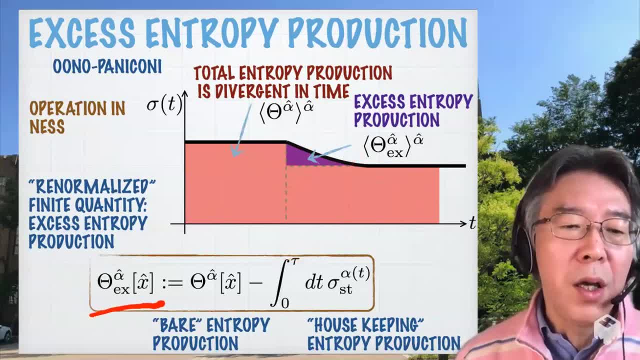 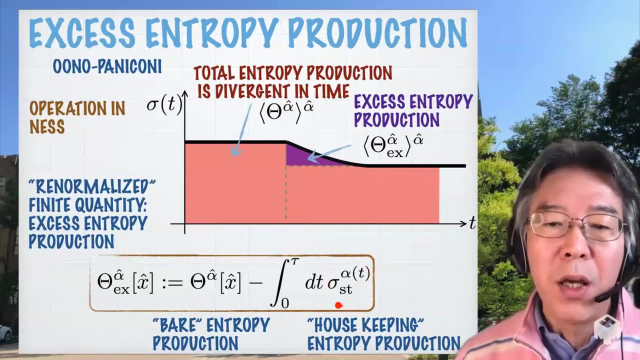 In general, this subtraction can be written in this way. So this is a bare entropy production which is divergent Here. this is the entropy production that we expect. So sigma s t alpha is the entropy production rate in Nes in a steady situation, with parameter alpha. So 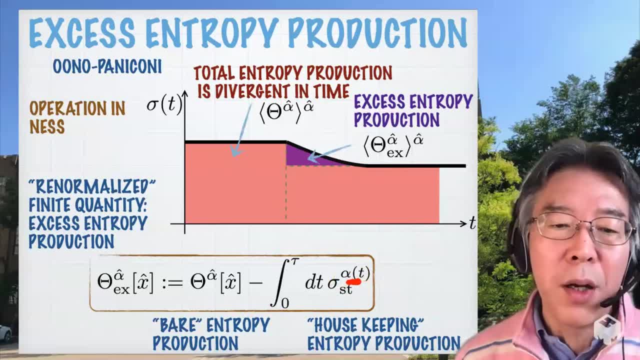 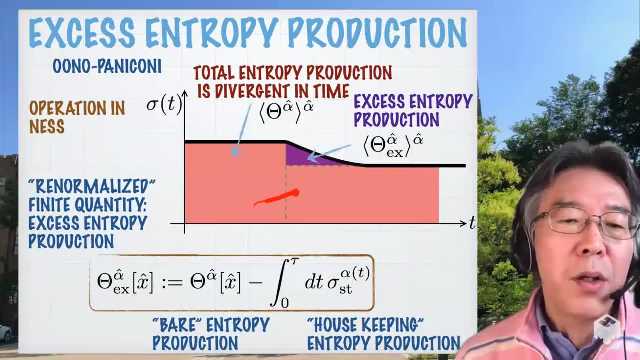 this is the entropy production rate that we expect from the parameter alpha t. So we simply integrate this and, you know, subtract this is this pink part, is this okay? and then you are left left with hopefully finite quantity. okay, so that's our renormalization. okay, this is a 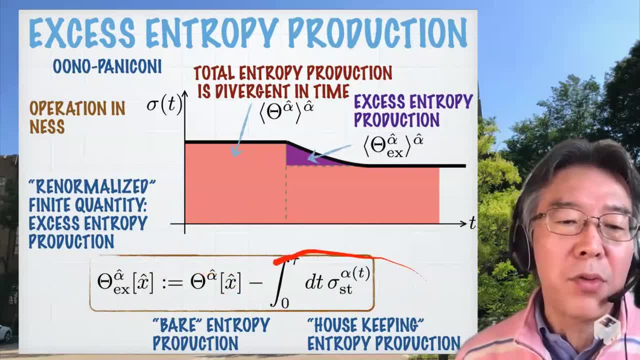 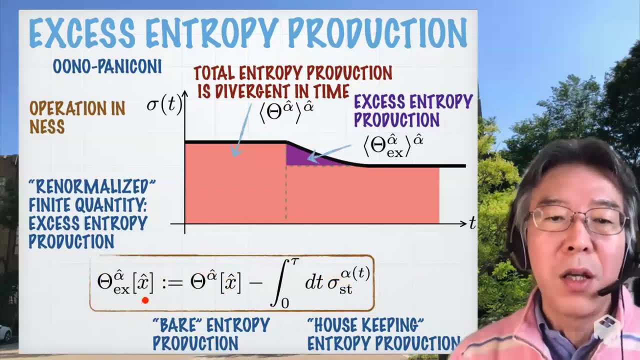 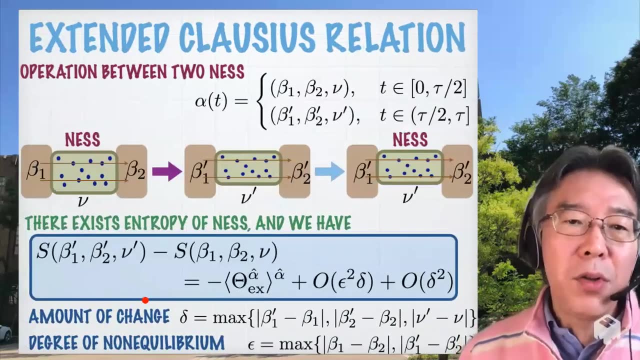 divergent quantity, you subtract another divergent quantity which you can determine from your parameter, and then you're left with this excess quantity which reflects the relaxation, relaxation process of the system, and then, yes, we do have extended closest relation. so this is our protocol. we change parameters suddenly and then we say that there is a certain, there is certain. 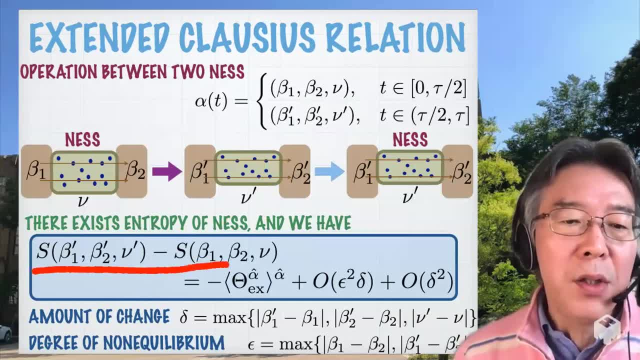 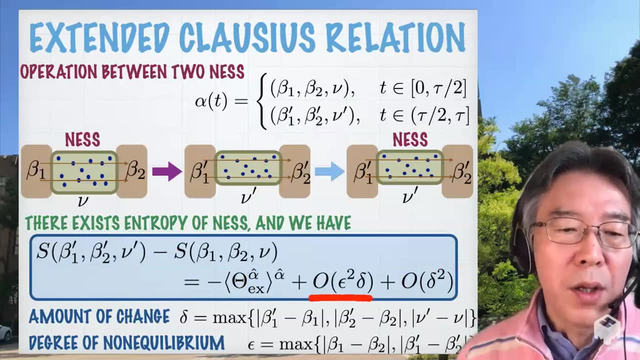 function non-equilibrium entropy and their difference is basically equal to the minus of this excess entropy. production, renormalized finite quantity. there is some error term- this is familiar error term coming from the step protocol, but this is new one- and here epsilon is the degree of non-equilibrium, basically the difference in temperatures. 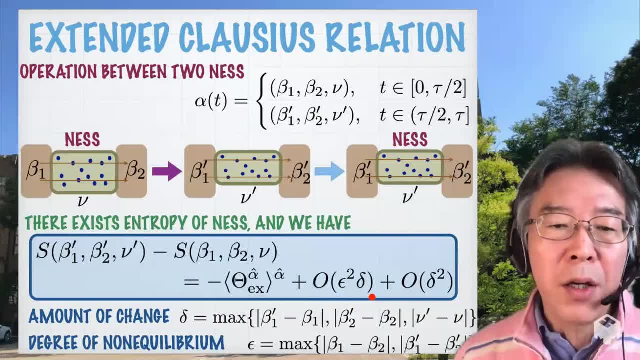 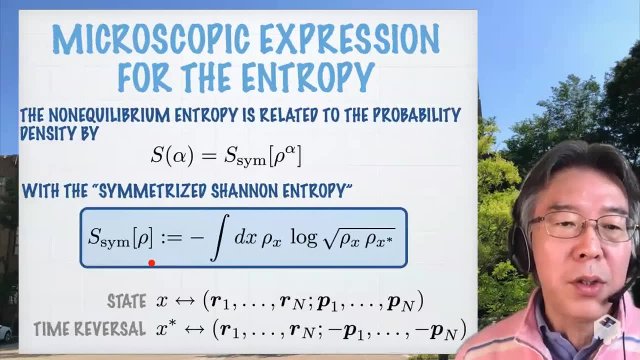 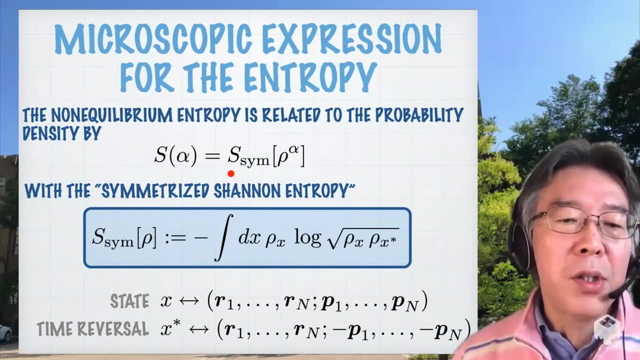 okay. so, uh, here, so this is vanishing in equilibrium situation, but we do have this, okay, and so what is this non-equilibrium entropy? that's interesting. uh, it's related to the probability density by this relation. and what is this? sm? sm is something very similar to the. 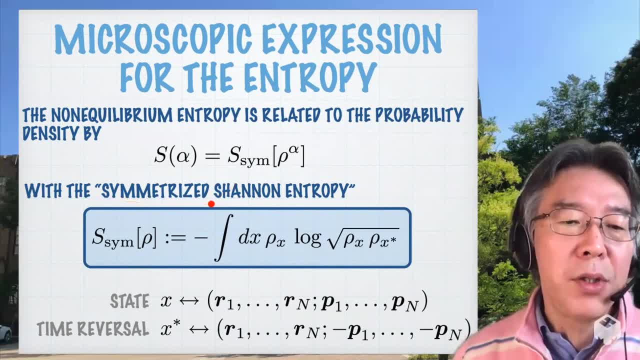 shannon entropy, but with extra symmetrization. okay, in shannon entropy we had simply rho x, log, rho x, but here we have this non-equilibrium entropy. and we have this non-equilibrium entropy. here we have square root, rho x, rho x, star. this is simply the time reversal, time reversal. 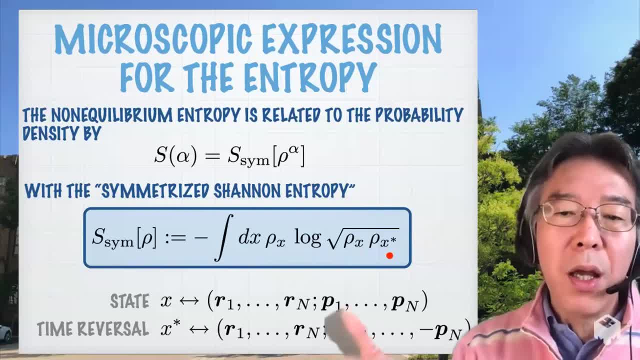 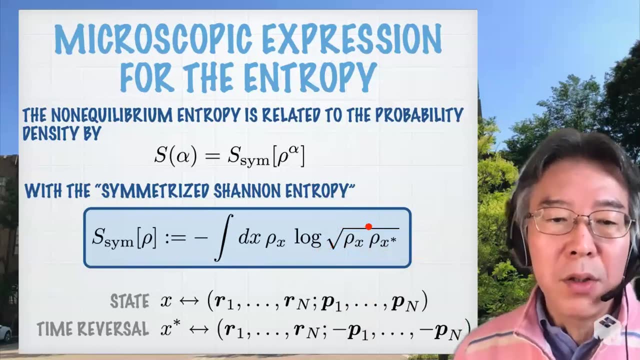 of this probability density and recall. in equilibrium, the probability- uh, equilibrium probability density, that is the canonical distribution- is invariant under time reversal. so in that case rho x star is rho x, so this square root thing doesn't matter. but in non-equilibrium case this does matter, and so without this square root thing, 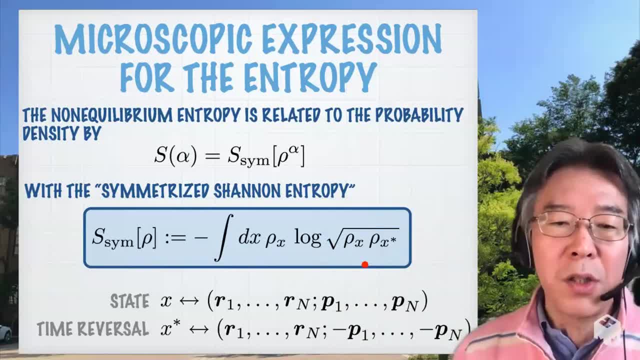 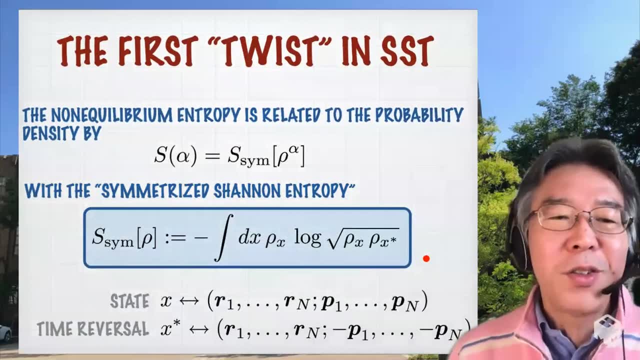 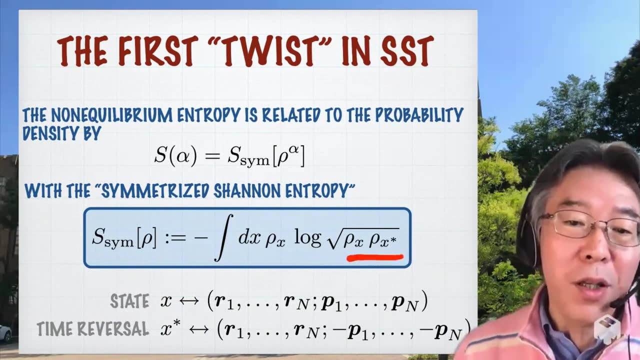 it's with only shannon entropy we never get extended clauses relation and with this, with this twist, okay, so this is the first twist. thank you for waiting. this is the first twist. instead of using shannon, we have to make this small but very suggestive twist to make this. 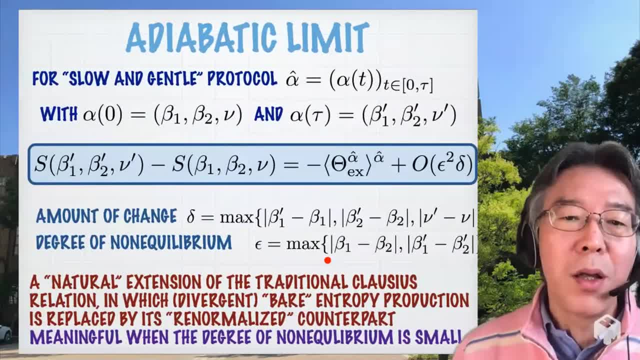 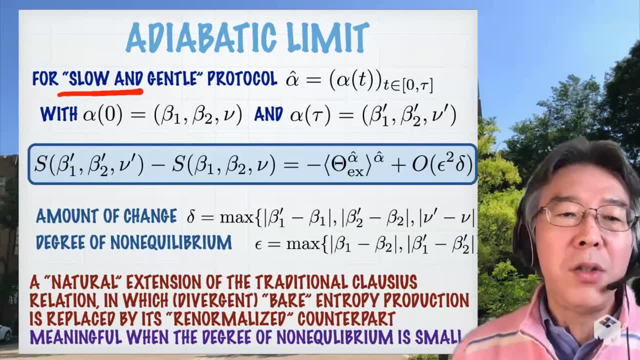 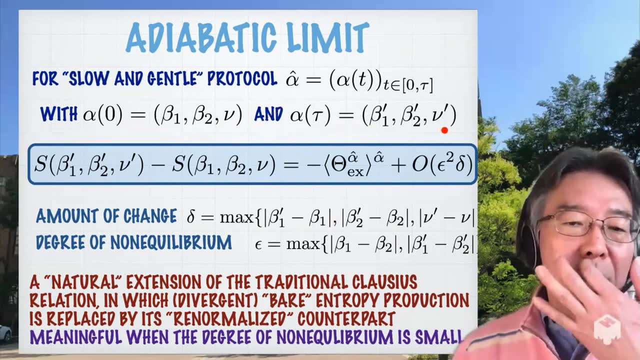 uh, extended clauses relation possible, okay now, uh, it's just automatic. but, as usual, we can extend. we can think about slow and gentle protocol alpha, which changes slowly and smoothly and it connects this value and this value and in this case, uh, our extended clauses relation becomes like: 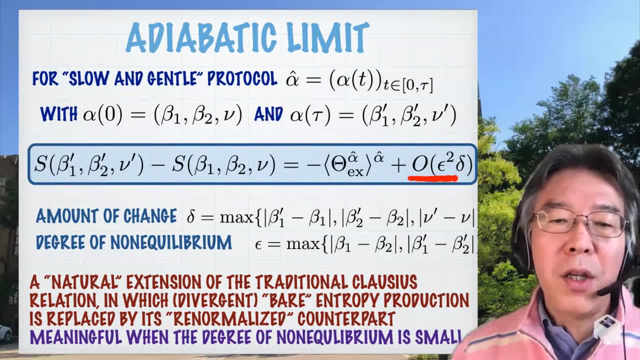 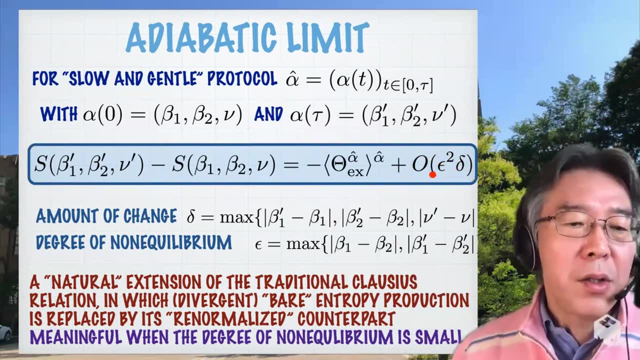 this and uh, unfortunately here we have this term. so if epsilon is zero, this is not here, so it's just usual clauses relation. but now we are in non-equilibrium situation, so we have this error term. okay, so here, anyway, we have a natural extension with the traditional clauses relation, in which 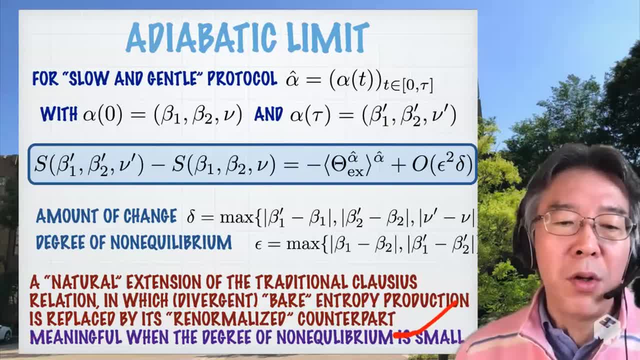 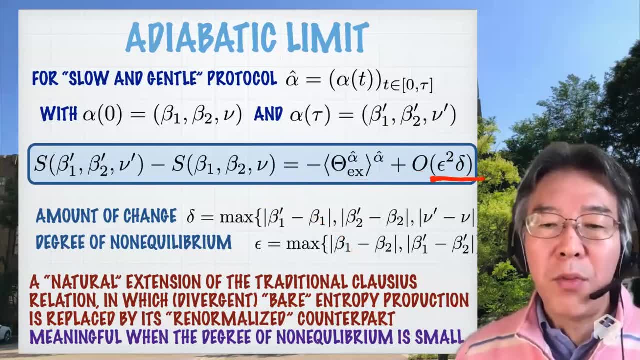 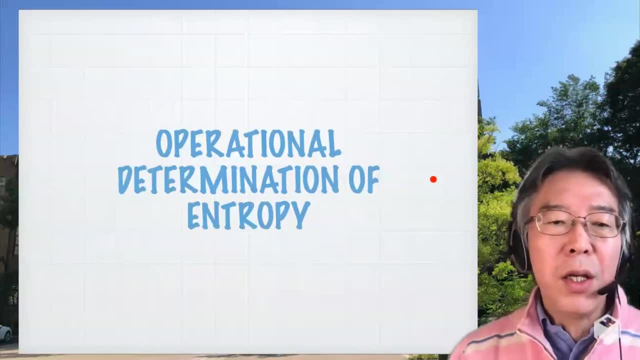 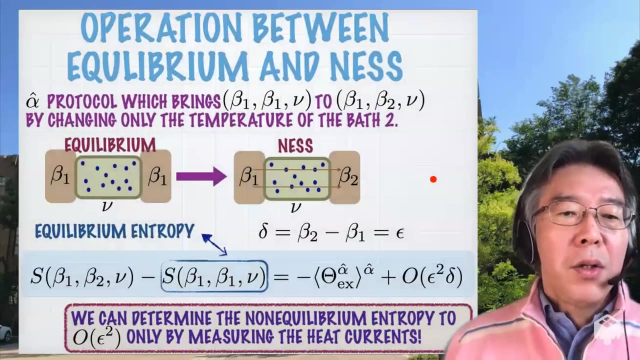 divergent bare entropy production is replaced by its renormalized counterpart, the excess entropy production. and, as i said, this is meaningful only when epsilon is small. so we have to be close to non-equal, close to equilibrium. now, with this, uh, we can think about operationally determining the entropies of ness. so first, 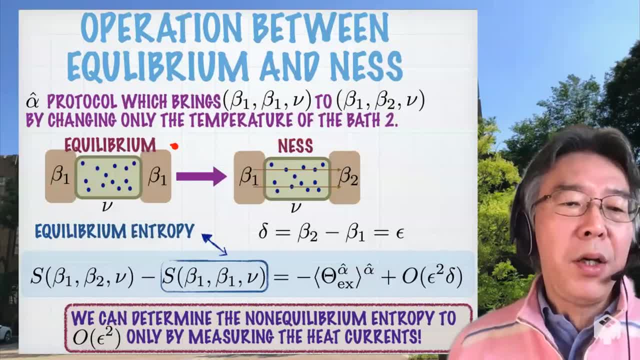 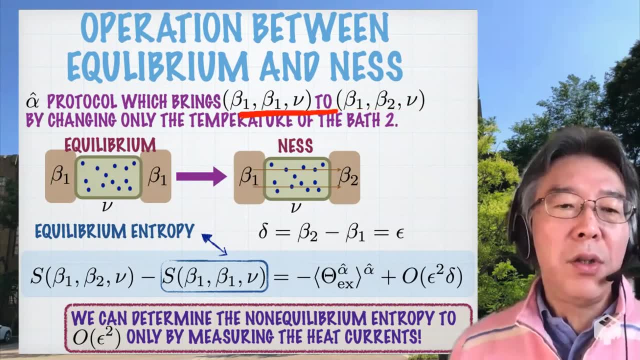 of all, uh, let's think about, uh, an operation which brings equilibrium state into a non-equilibrium state, like this. so to realize this, you simply fix beta 1 and nu and only change the temperature of this right heat path from beta 1 to beta 2. and here i can use, and slowly, gently, okay. 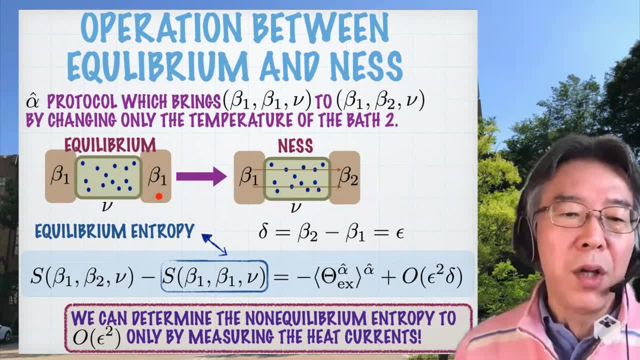 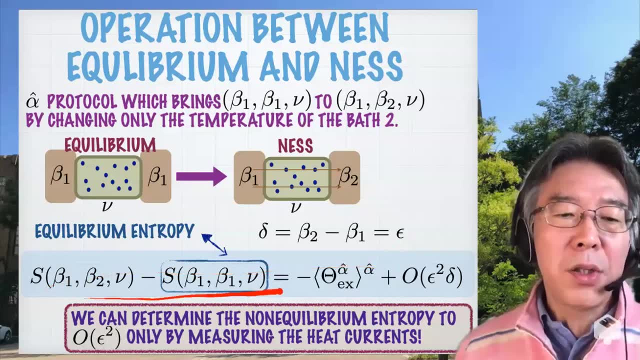 you change this temperature slowly, gently, to beta 2, and then you start from equilibrium and you end up in ness, and in this case, uh, this is our extended clauses relation. but in this case, uh, delta, the change in the parameter is basically epsilon, so this error term becomes order: epsilon cubed. 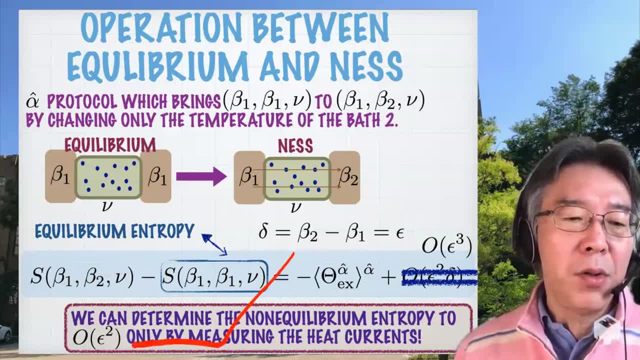 this means we can determine the non-equilibrium entropy to order, with the precision epsilon squared, only by measuring the heat currents. that means: uh, this thing here is in principle, uh thing here can, it can be in principle determined by measuring heat. right, uh, you just draw this and 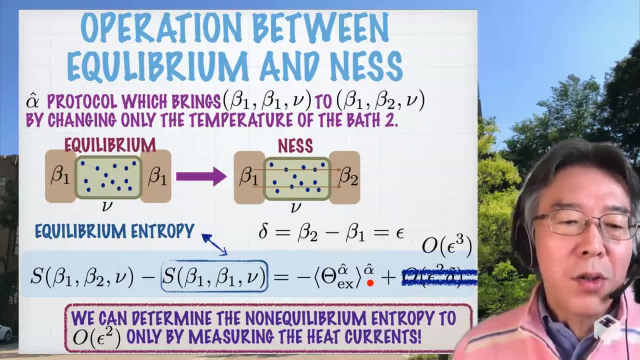 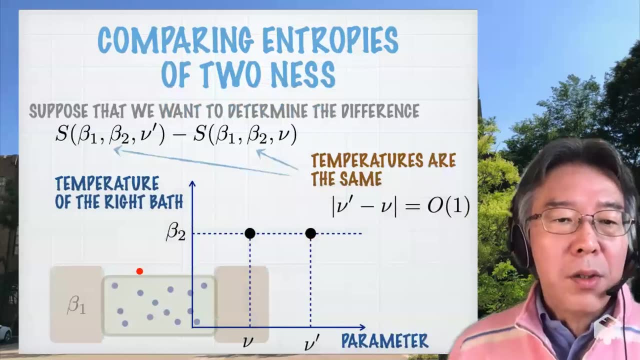 you just subtract and you know so, integrate and so on. so, uh, this tells you that by, by doing this experiment and measuring heat, you can determine, determine this difference, and of course this is a equilibrium entropy. so you know this, so you can determine this thing, okay, next, uh, let's think: 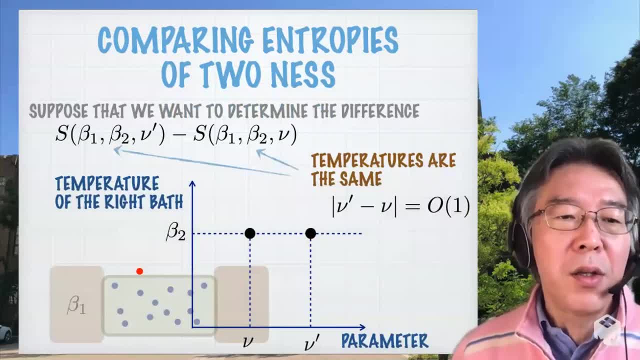 about comparing entropies of two nests. okay, so now i fix beta 1 and beta 2. okay, and they are different. and now i think about changing this new, like the volume or external field. so, uh, this is a okay, this here. here i have fixed the temperature of the left west to beta 1.. and here only i did. 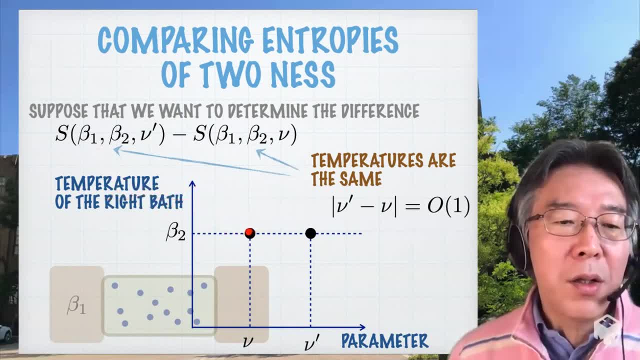 depict temperature of the right path. but here, uh, the temperature of the right part are the same, and so, and so here i fixed: the temperature of the right part the same, and these two are the same. so, and I only change the parameters, And I want to compare the entropy here and here. okay, 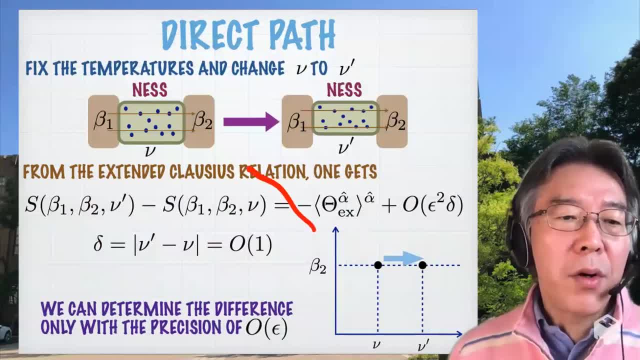 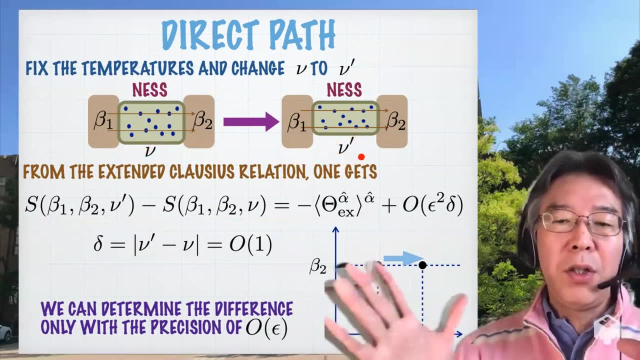 And now, if we use our extended Clausius relation in this situation? so I gently, I fix two temperatures and I gently change nu from nu to nu, from nu initial value to nu prime, Slowly change the volume or slowly change your external field. 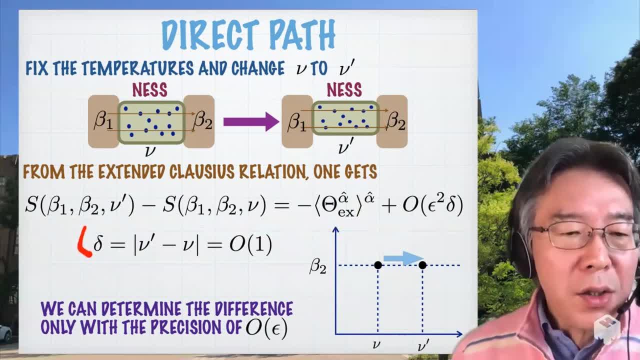 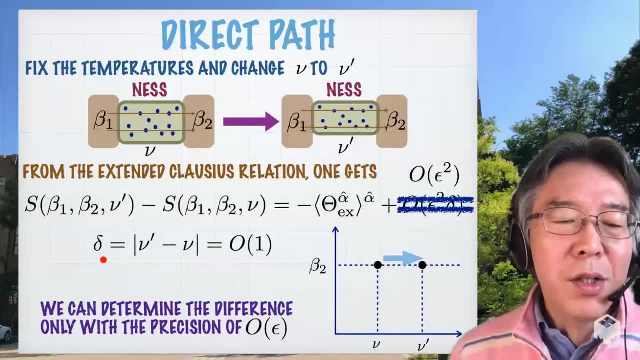 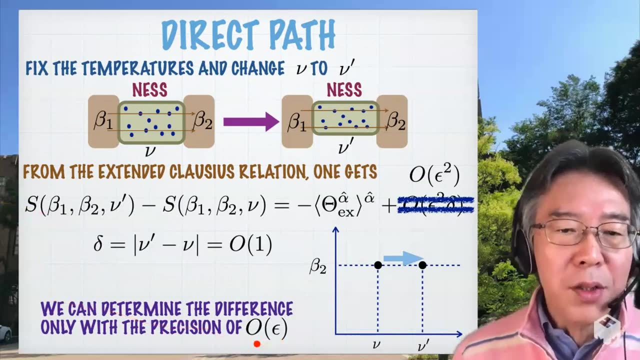 And then we have this relation, But in this case delta is of order one, So this LR term becomes order epsilon squared. So this means that we can determine the difference, but the precision is simply order epsilon. That's sad, But we can think about doing something else. 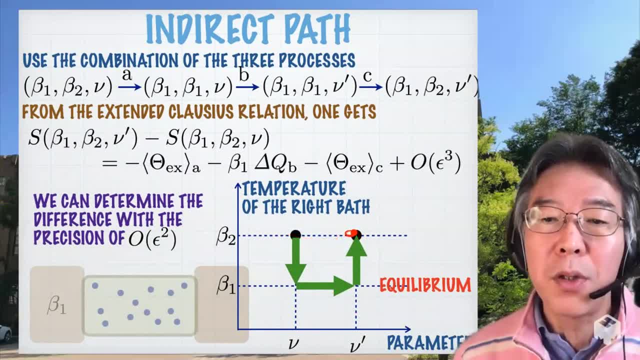 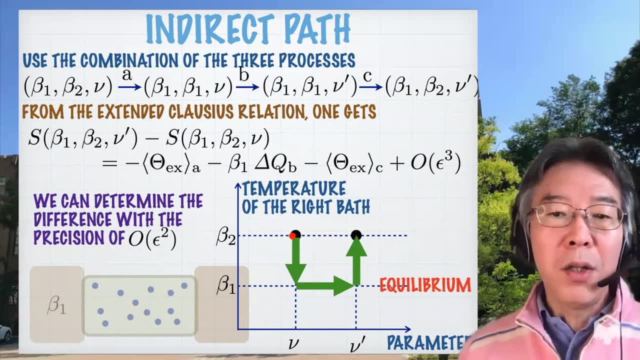 So we want to get to compare this point and this point And we first thought about going here to here directly. But instead you can take an indirect path. You start from here and go here first, and from here to here, and from here to here. 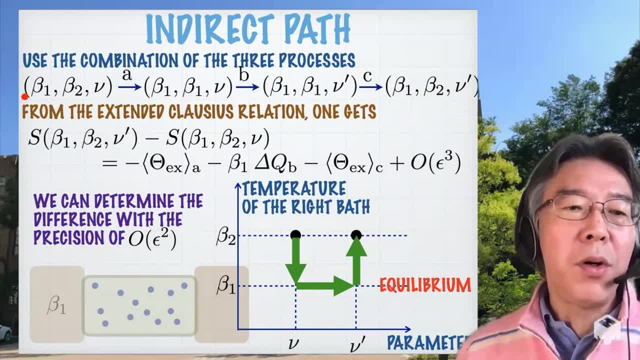 So this is here, and then you can use first of all our extended Clausius relation here and here. this is the equilibrium. This is just a usual equilibrium Isotherm operation. So you can use your Clausius relation, and here you use our extended Clausius relation. 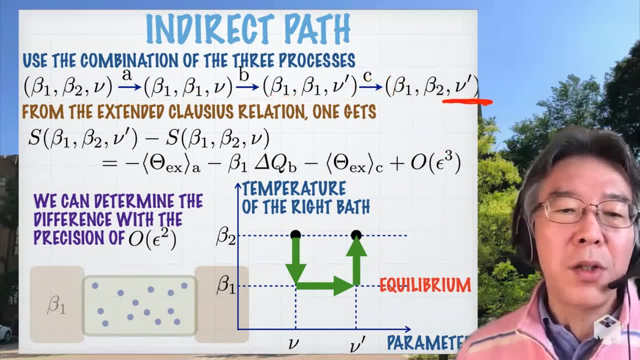 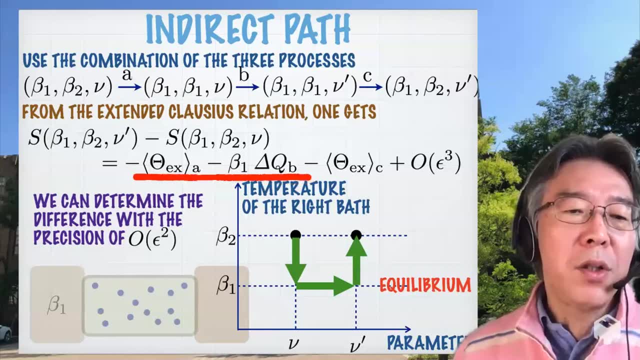 between equilibrium, no, no, between equilibrium and this, and in this case, uh, what we get is this. so, here again, these are the quantities you can determine by measuring the heat current. oh, no, no everything. yes, these are the quantities that you can determine by measuring heat. uh, heat. 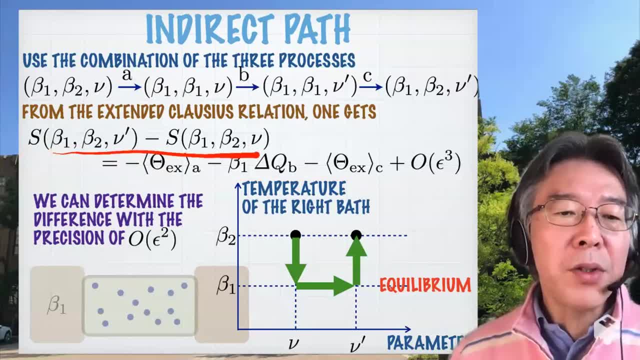 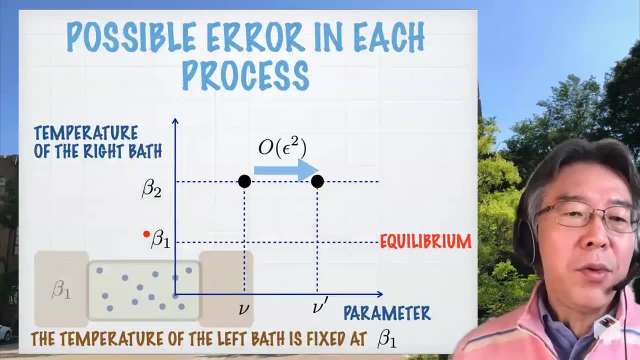 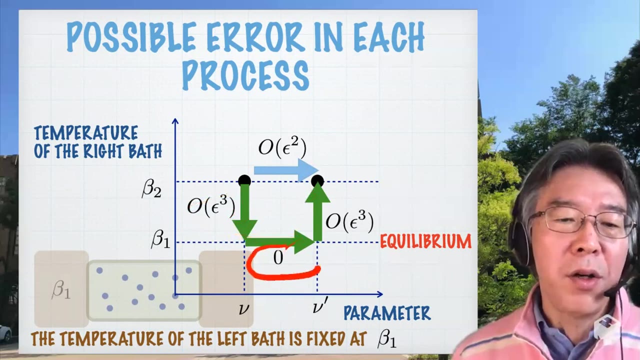 currents and we can determine the difference in entropy with higher precision order epsilon squared. so to summarize, uh, possible errors in each process is: uh, if you go directly, that error is possibly order epsilon squared, but if you go in this way, uh, error is smaller here, here and error is zero here. 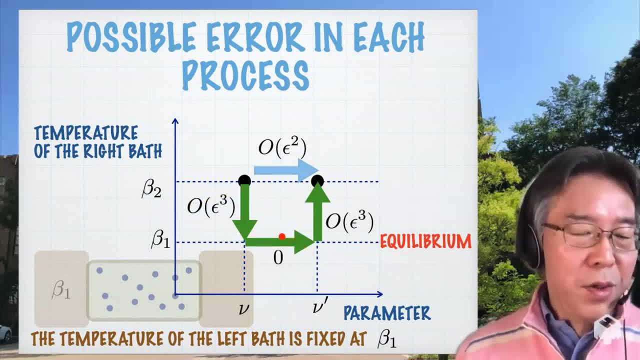 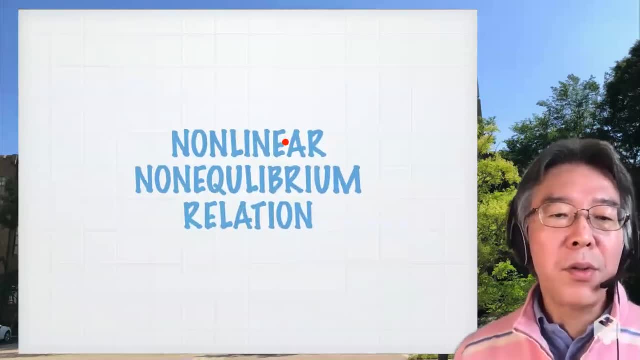 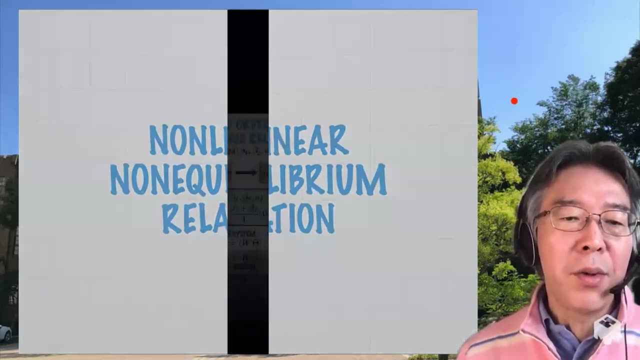 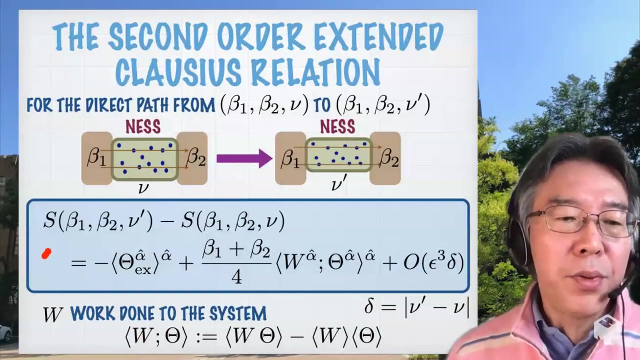 okay. so this is a bit weird. so you of course ask: can we do better here? and yes, we can. so we are coming up to the almost to the final part. so i'm going to talk about new non-linear, non-linear, non-equilibrium relation, and actually we can. yes, uh, we can prove a better, improved extended clauses relation type. 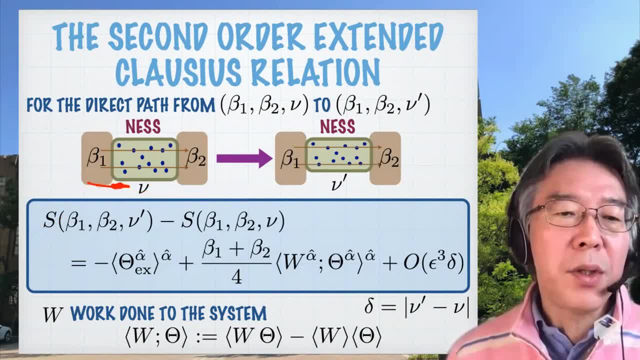 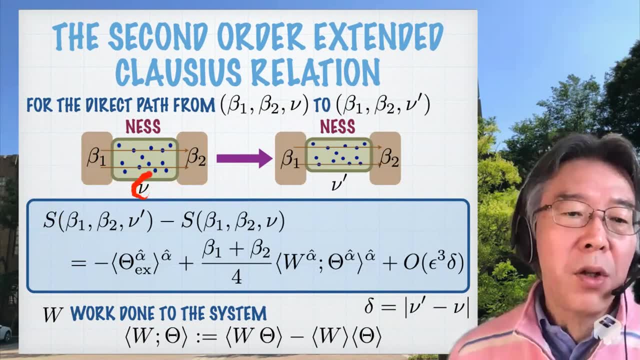 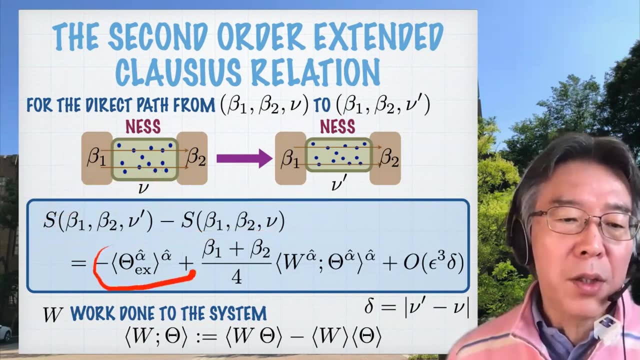 quality for this particle. you fix temperatures- b1, theta, beta 1, beta 2- and you change nu, like the volume or external field, slowly, gently, gently, from nu to nu prime, and then this is valid and then this is valence, as we have seen. so we can say that we are going to have a good 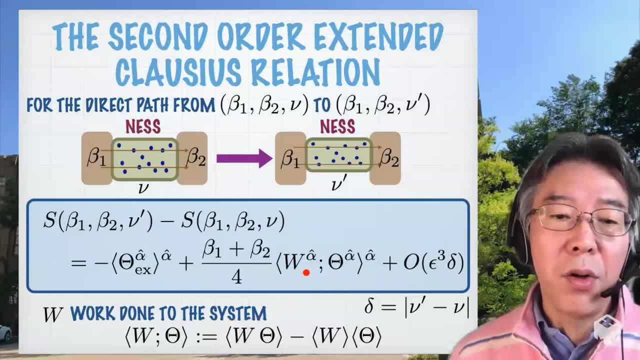 follow-up of the same non-equilibrium entropy, the same excess entropy production, and something new here. w denotes the work done to the system, the work done to the system during the whole protocol, okay, during the whole operation, and theta is of course the total entropy production in the bath. and 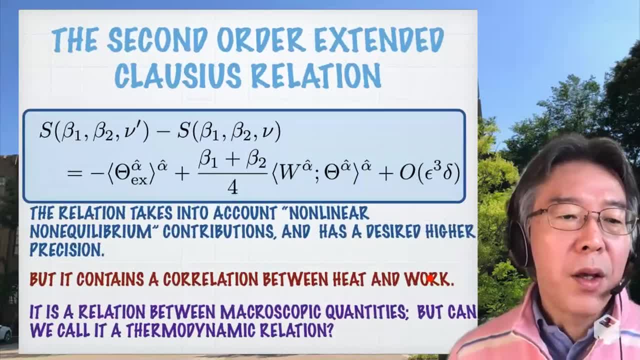 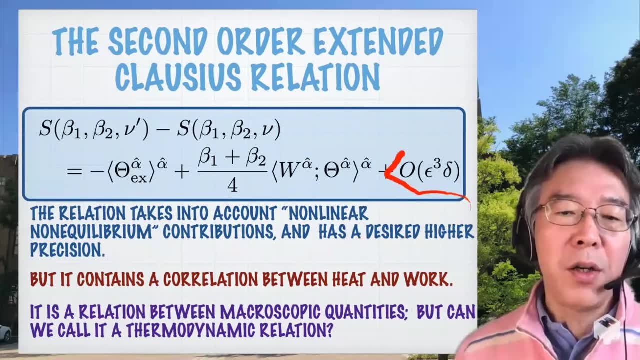 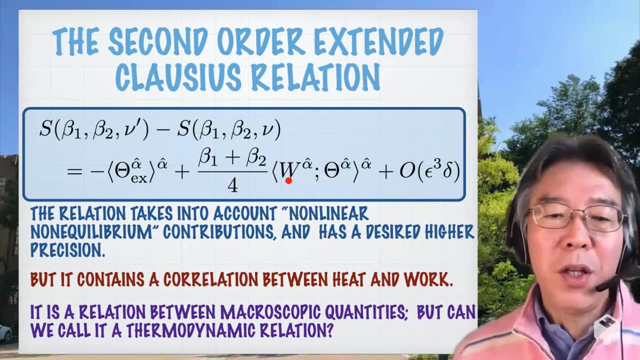 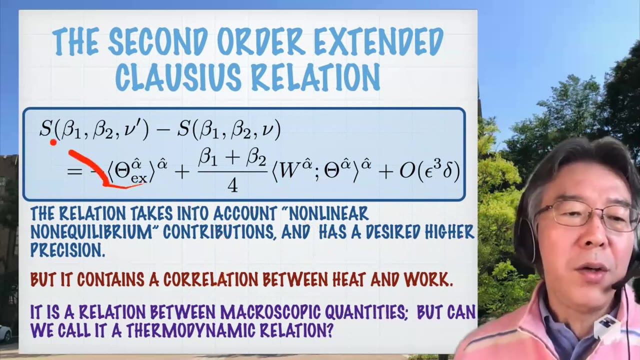 this has a higher precision. so this relation takes into account non-linear, non-equilibrium contribution and it has a desired higher precision. that's nice, but it contains a correlation between heat and work, okay, so anyway, it's a relation between macroscopic quantities we only have. so 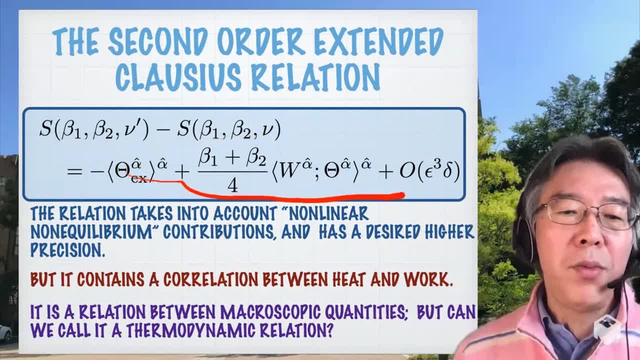 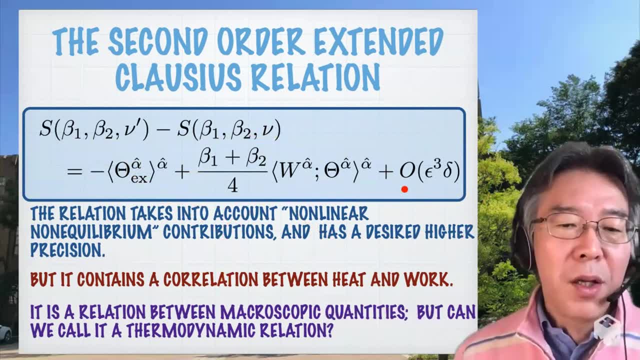 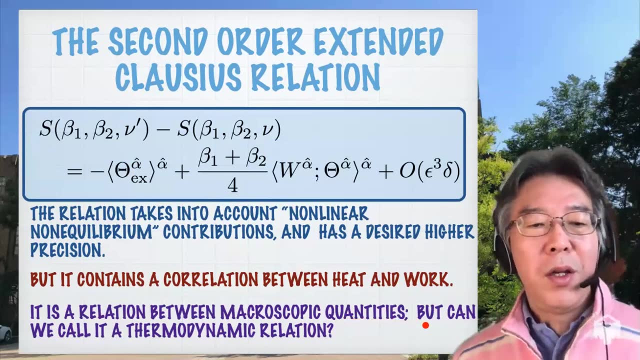 these are macroscopic entropies, these are all macroscopic quantities. i mean, they can be determined by measuring heat and work, okay, but uh can. but, but you know, uh, it only contains a macroscopic quantity. but can we call such a such a relation containing correlation of thermodynamic? 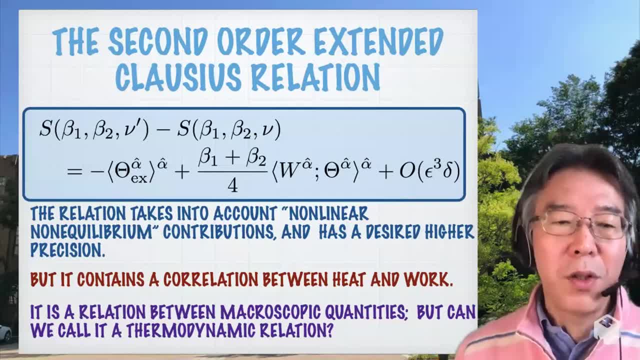 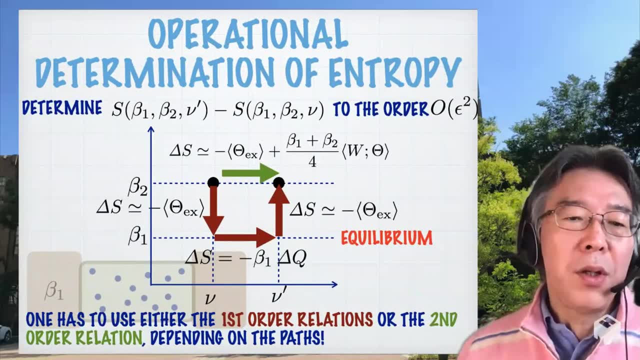 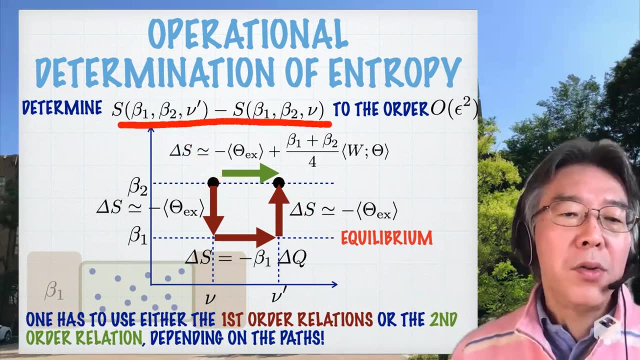 relation. uh, that's something we don't know, we still have to think about. and now? so this is a summary for the operation- dimensional determination of entropy. So suppose that we want to determine the difference of, yeah, difference of this- two non-equilibrium entropies. 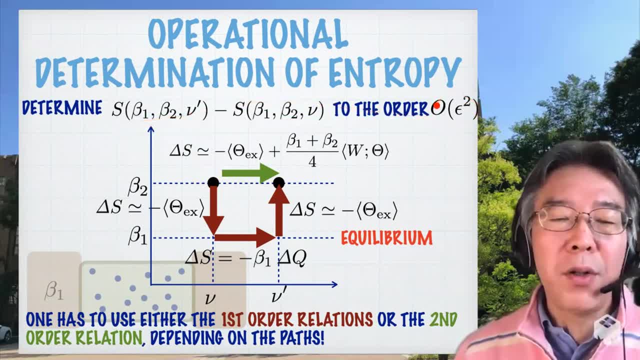 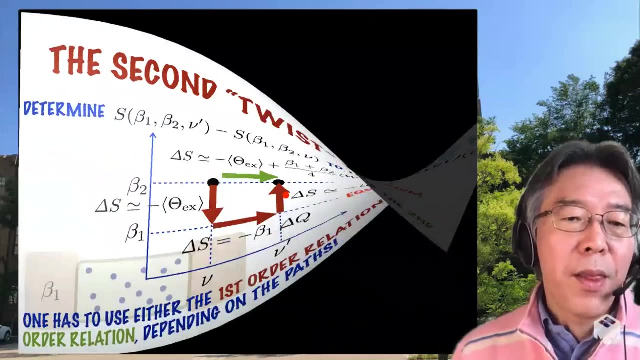 to the. with a precision order epsilon squared, then you can do it, either going directly from here to here, or you can go from here to here indirectly, like this. But isn't this a twist? Because in order to get this same precision,